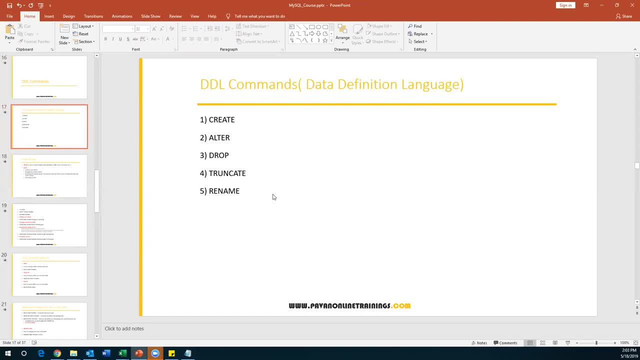 Modify the column. Okay, I want to delete the column of the table. So these things we can perform By using DDL commands. so create, alter, drop, truncate and rename. So these are the five commands which come, which are comes under data Data definition language. Okay, So now we will see how to use this particular command. 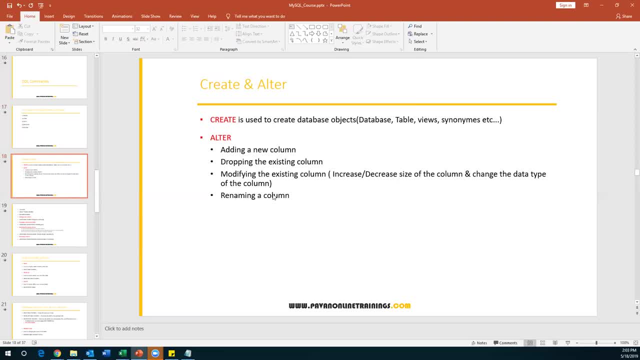 The first command is create and alter. so create is creation, So it will create a new database object. like it can create database, You can create a table, You can create a view, we can create synonym, So not only table, So we have multiple type of objects. 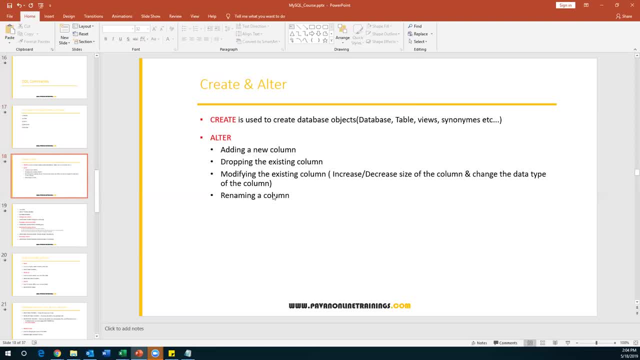 or there in the database. So, but table is a very basic entity or basic object in the database. So we have also use, you know name, So these are also there in that database. We'll see them later. So basically, the create is a command by which we can create a new object in the database. 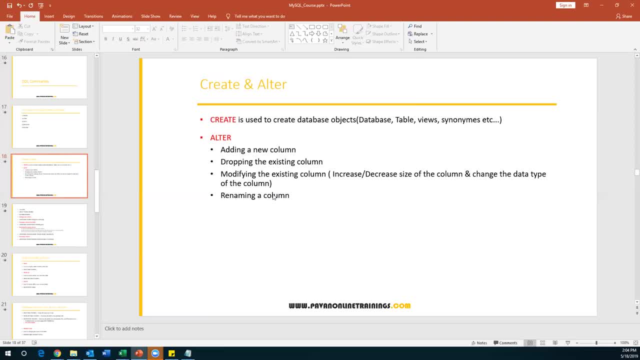 New object, in the sense It can be database or schema, or it can be table, or it can be views or in the scene and whatever. If you want to create something new, we have to use a create keyboard, and if you want to modify something- or suppose I already- 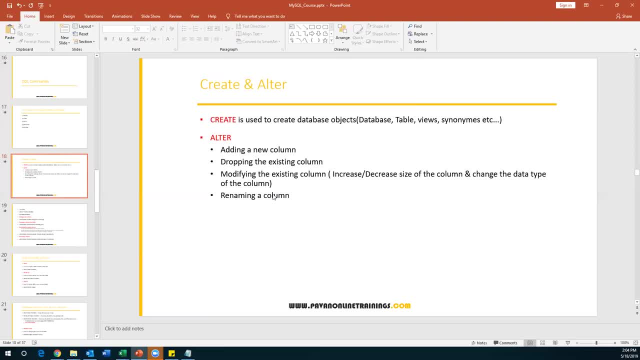 created some table. in that particular table, I want to add a new column and of, or else I want to drop the existing column, or I want to modify the existing column with respect to size as well as data type, or I want to rename a column. so these things are possible by using order command. so create and order. so now. 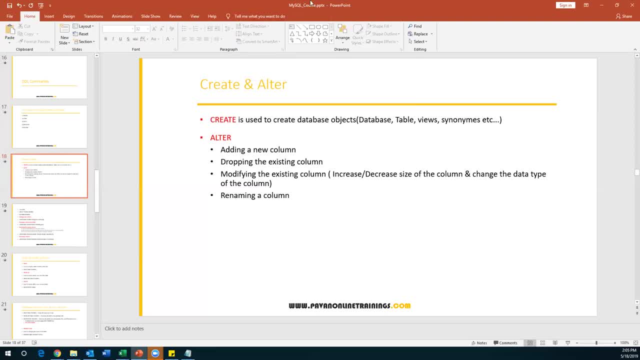 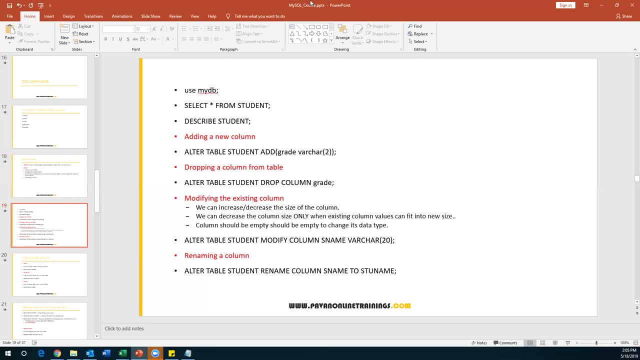 we will see how we can use this particular command create an order. so here I have few number of queries. so we have a student table in the my DB we created in the last session. so in that particular table I'll show you how we can use this particular command create an alter command. okay, so let's go to our 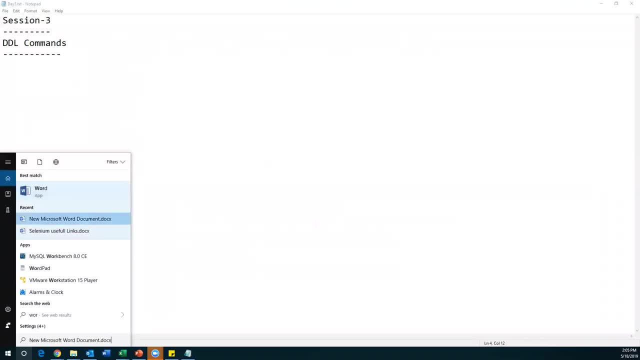 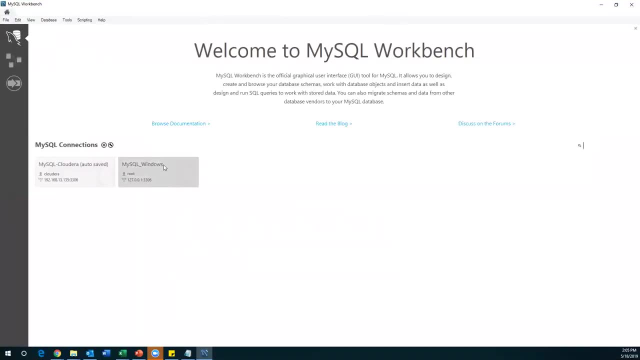 workbench client. so let me show you this is my workbench client. let me open this. so once the workbench is open, we need to. this is our connection, which is already created earlier. so I'm opening this connection. just click on this and now it will opening the connection to the database. 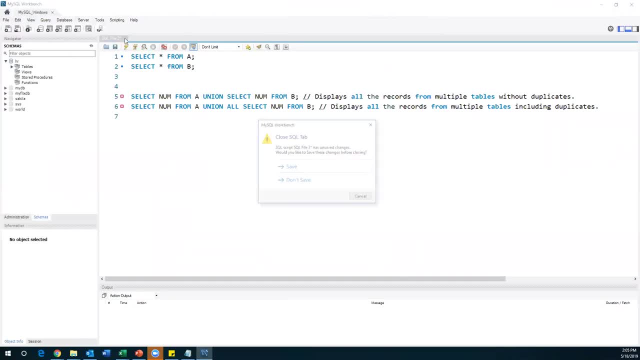 so now I'm just reading or remove this, so now I have schema. so these are the current schemas are available. so currently we are working on HR and as well as my DB schemas right, so now I'll go to my DB schema. so here I have some. 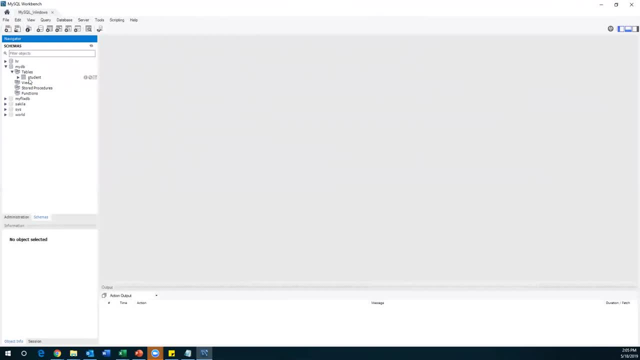 student table. I'll first delete the table and then I will create a new table by using create command, and then also I'll try to alter some of the columns and names, all these things. so first of all, let's open the query editor. so if we click on this option, so here it will open the query editor care. 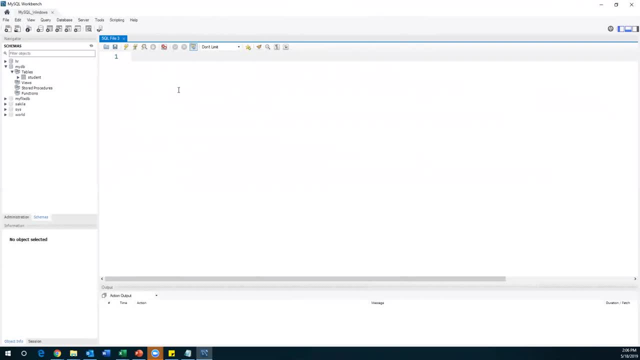 so how to delete the table? so how to drop the table is: we have a simple command call. first of all, we need to use, use HR, use my DB, so it will go to our deep database. let's Ord this command and then now it is focusing on my DB. so now, 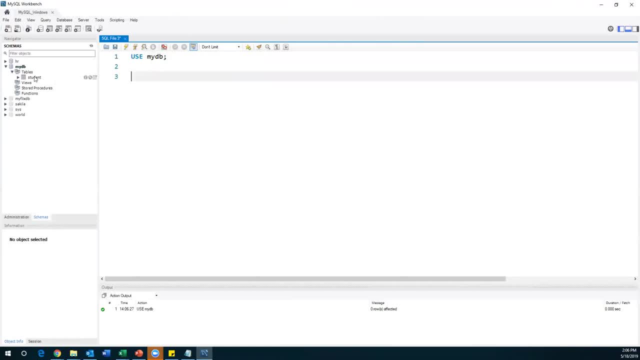 we execute this command. so, first of all, I'll drop the existing student table and then again recreate this. so I'll just say: Ukrainian, commissionerdermabase, gambt, malaycom, Drop table student. So this command will drop the complete table along with the data as well as structure. 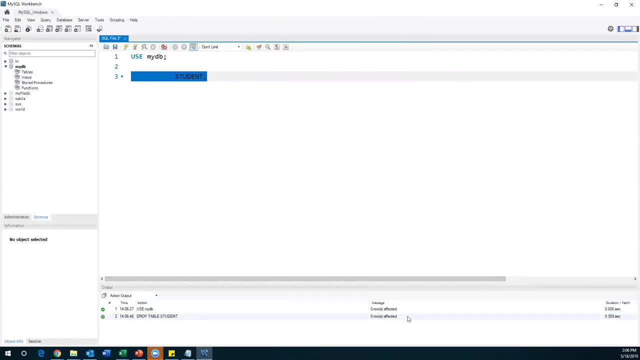 So when I execute this, so drop table, student is done. So when I refresh your project here, so click on the refresh now, student is gone. So I don't have any tables in the my DB. So now I'm going to create a new table. okay, so I am going to create a new table in the 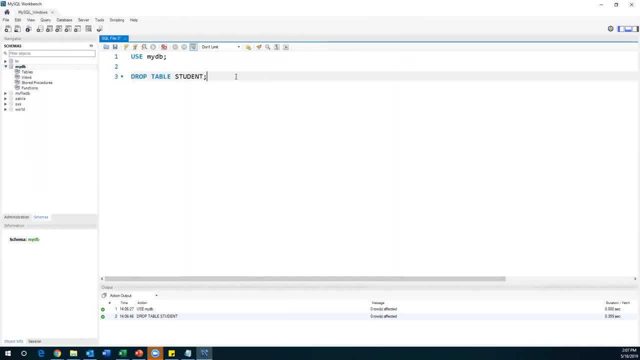 My DB database. so how to create the table? So command is create. by using create command We can create the table. So create table student. and Here we need to specify the columns. I'd say SID, SID and say integer type of data. So I have said four pages I need to have 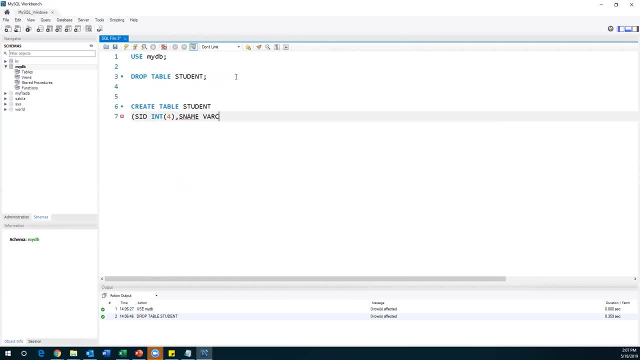 Comma s name, that's the student name and this is a string type of data. I'll say, And I will allow the 15 digits or 15 characters and S name and say SID s name and Currently we have only two columns, So one is SID and S name. 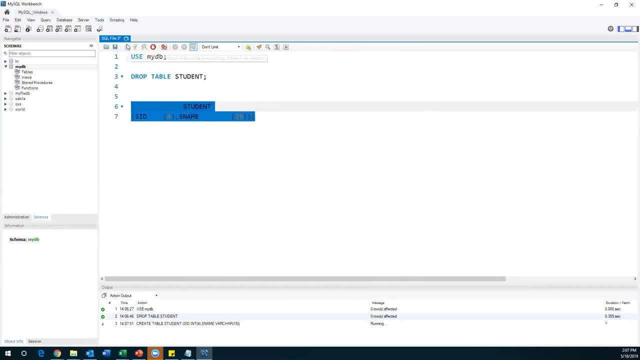 So now execute this command. this will create a new table in the database. now that new table is created, So refresh here. So then you will see the student table. So once you describe this table, let's say describe student, and This command will give you. 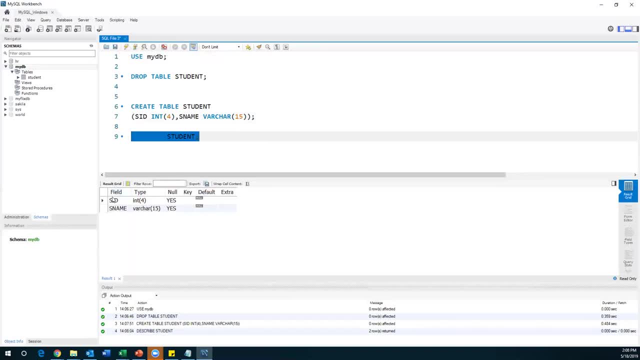 Whatever columns and available in this particular table. So currently we have only two fields and the type of the fields, and the nulls and the row. There are no other information is available. Currently We don't have any data in this table. Fine, So now I'll try to insert some data. 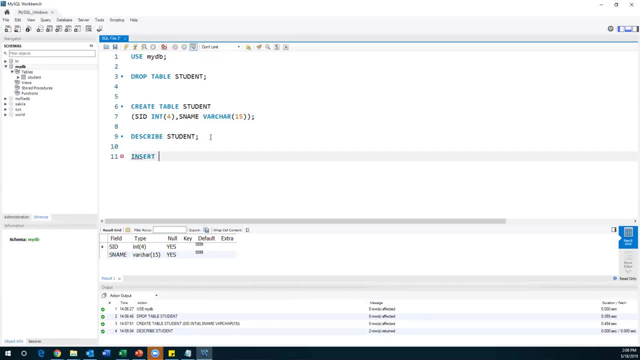 So let me insert our two records. Let's say how to insert data. insert into student. there's a table, name values and SID is a number. So I'll just say one, zero. one S name is a string, So Put in the single quotations. So here I will say David. So this is a first in the statement. 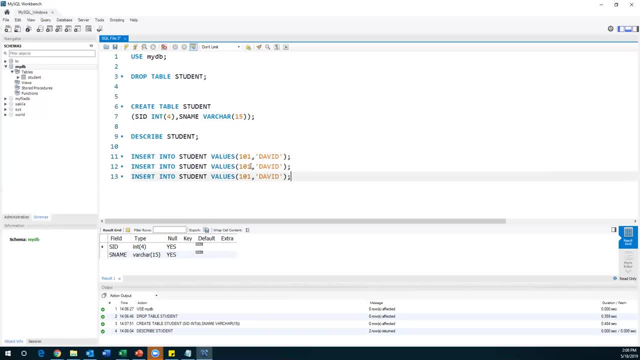 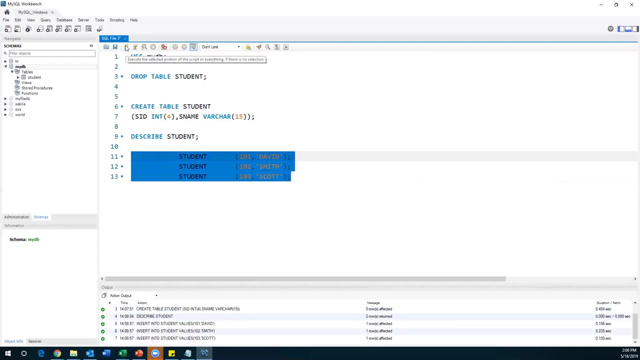 I will also insert a few more records. Let's say, this is two and this is one three, and Here's Smith and He is a Scott. Okay, so let me execute all this thing together, all the commands we can execute together. So fine, So all the instance statements are successful, and now what I will do is I will exclude one command called 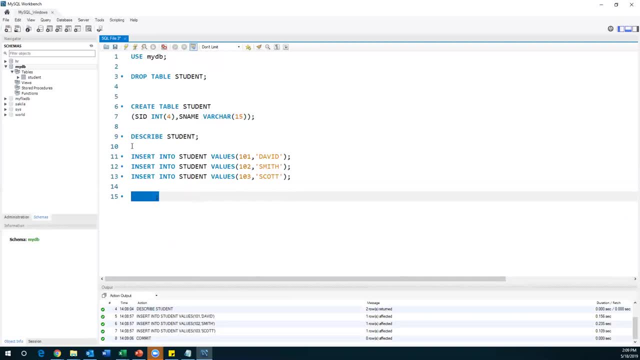 So until unless we execute this, come in, the records will not be perfect. Okay, fine. So now let's execute the command for retrieve the data. So there's a select a star from student and Execute this command, then we have a three records currently in the table right. 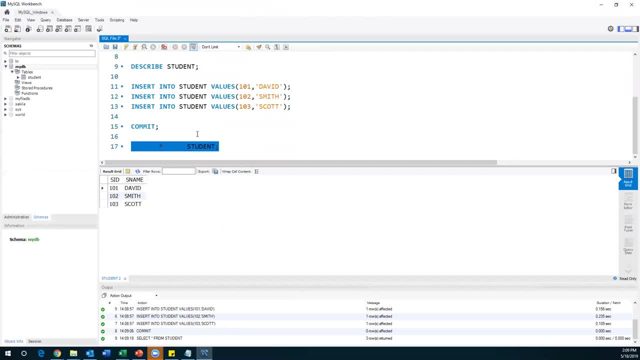 So, after doing all these things, suppose I want to alter the table Like: I want to add a new column in this table. I want to add a new column in this table, or I Want to rename a column in this table, or I want to drop the existing column in the table. 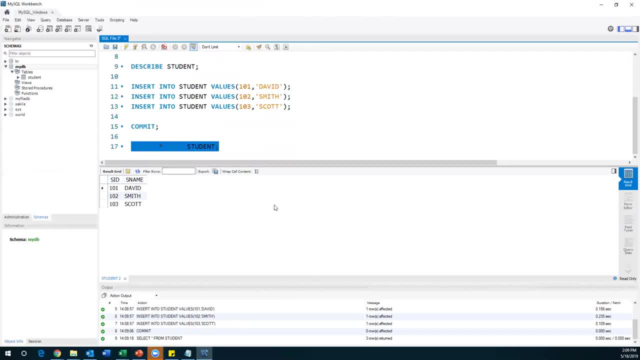 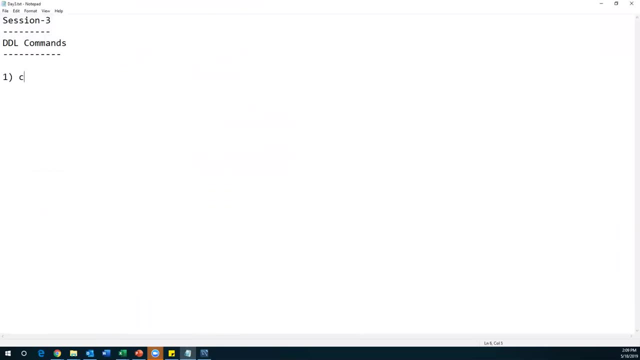 So to perform these things, we can use alter command. Okay, so we use order command, So detail command. The first command is create command that we have seen just now: create command. by using create command, We can create the database objects. now, by using alter command, We can alter the database objects. 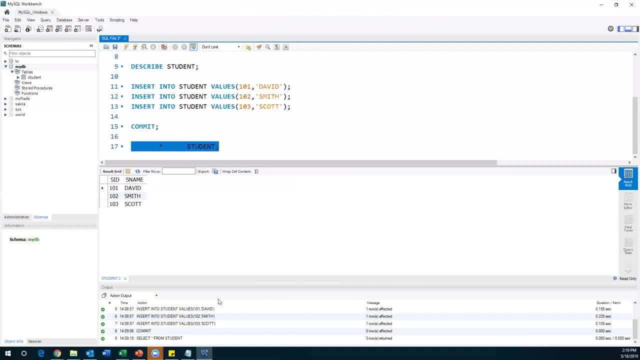 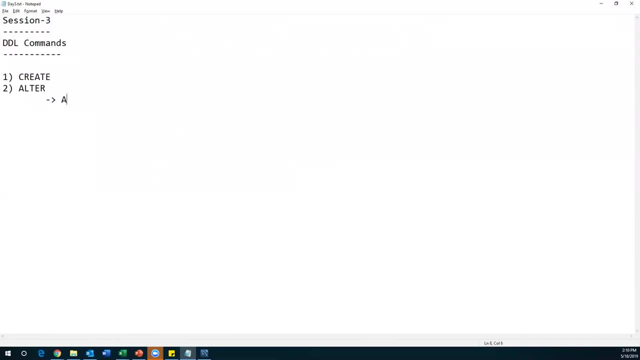 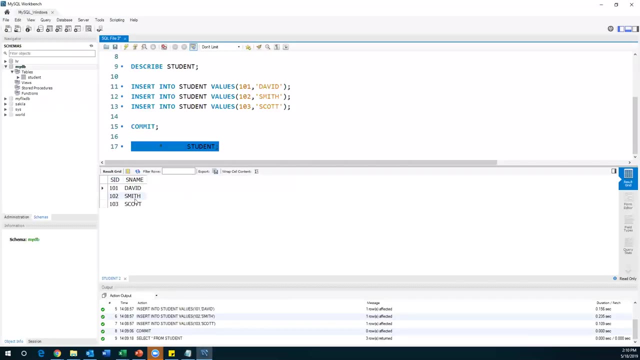 So now I'm going to perform few things. one is I want to add a new column. So by using alter command, I want to add add New column. add New column. so currently I have a two columns- SID and S name. So I want to add one more column called as a grade. So I want to add student grade. 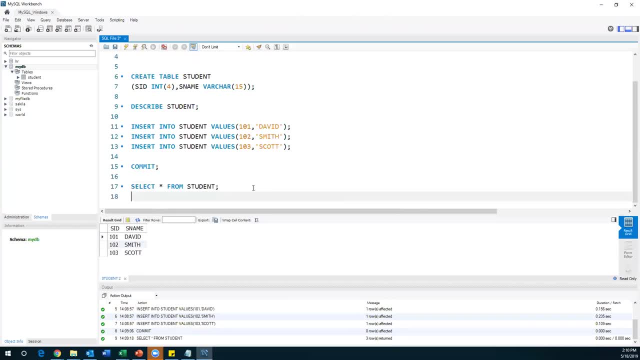 So how we can add that? so by using order command, so we can add like this: So command is alter, You can also type in small. You can also type in small letters All the commands, because sql is a not case sensitive. Okay, so alter. 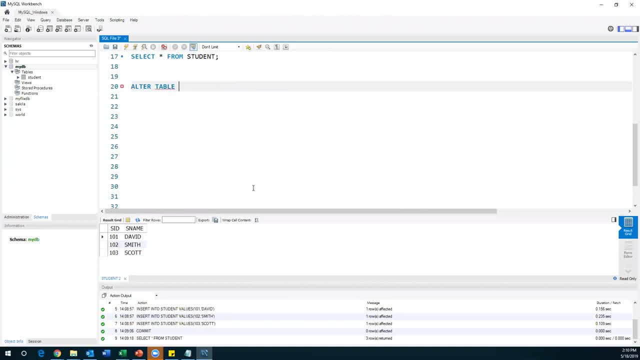 table, Alter table and table name. we have to specify so, alter table, Table name, that is, your student Alter table, table name, and we have to add the new column. So here we have to use one keyword called Add and which column we need to add. we need to specify the column name, data type and the size of the data. 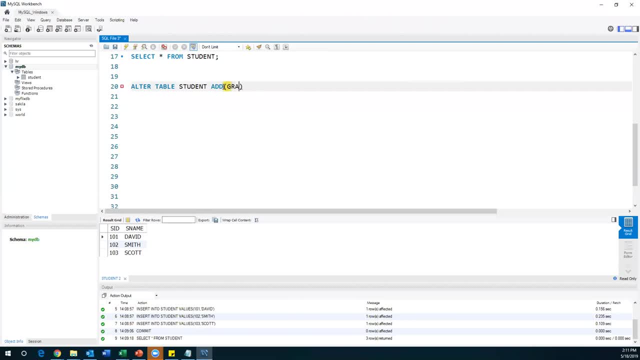 Type. suppose I want to add a great call. So here I'll say grade, and The type of the grade is, let's say, back I'll say two digits. I'll allow it, That's it. So now execute this command. So alter table student. add grade of this. 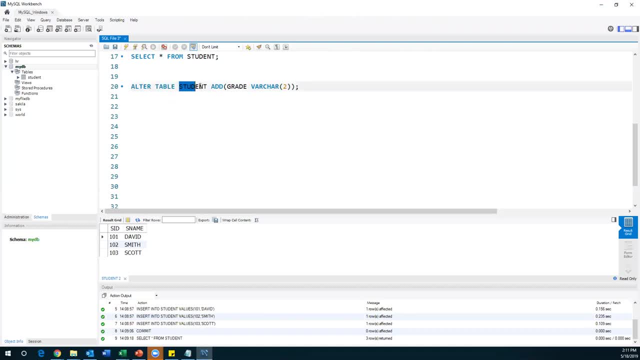 So this is a command: alter table, student add, and This a column and the data type and the size of the data time. So worker is a data type, So means it will allow the character type of data. So now I have just stated one statement. now let me execute this and 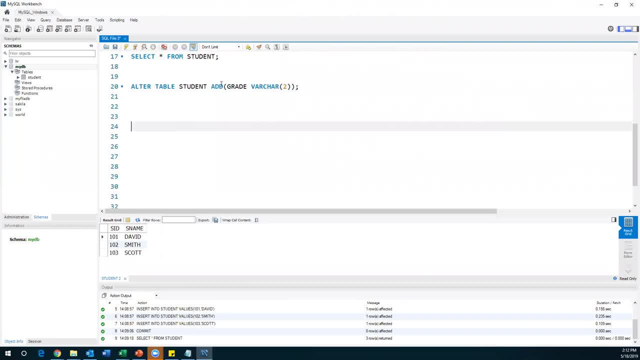 alter table: student is my student name. table add: Grade is my column and data type of that column and to me. So grade will be normally one single character, but I additionally have given one more character, So it will allow the only two characters, so execute. So now it is executed successfully. 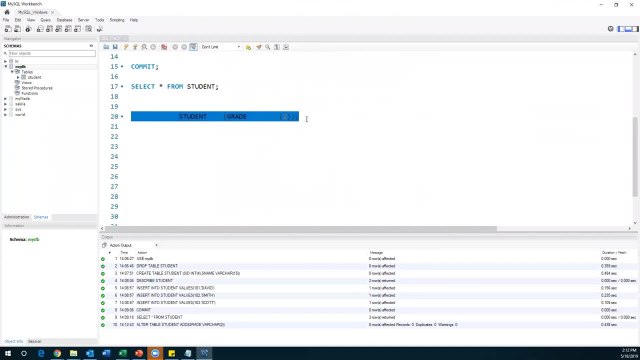 So order table student pad is executed. So once it is executed, if you want to see the structure of the table again, execute the describe command. so describe student. So once you describe the student now, it will give you another column. now you can see s id s name. grade column is added. 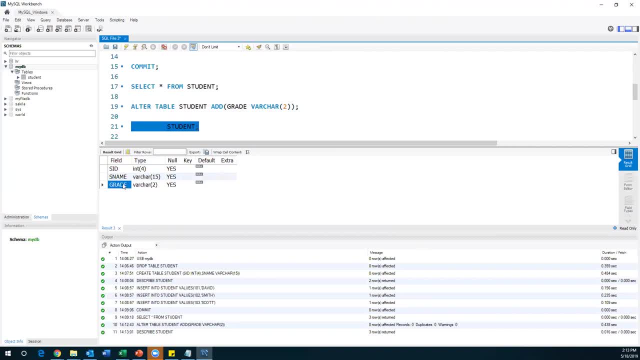 so s ID S name and create column is added, but at the time of inserting the data, we have inserted only as ideas and estimates, But we don't, we haven't inserted any create right, because this is a new column which we have added just now. but if I select this data from the table, what is giving it is? 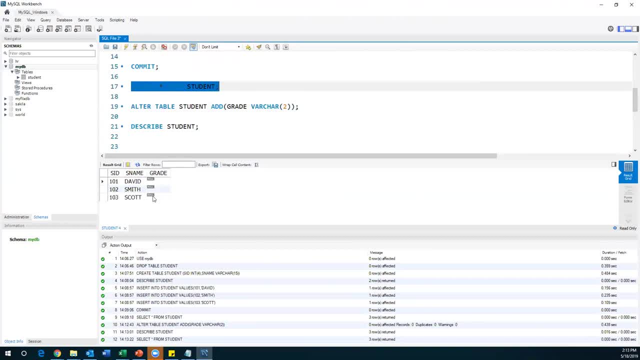 giving null. so these values we have not inserted so far, but SID as name is already have the data, but additionally have added the new column called as a great. okay, so if you want to update this particular column, you can still add that one. so we need to just use update commander. update grade is equal to, so 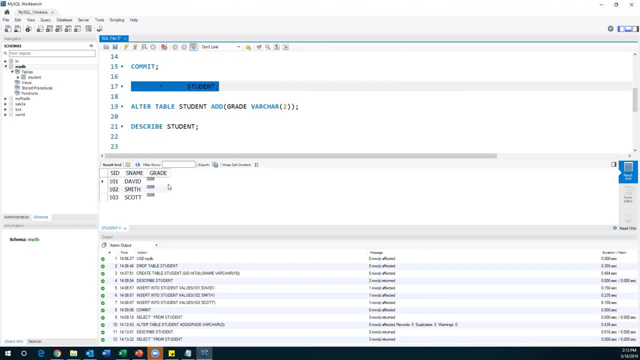 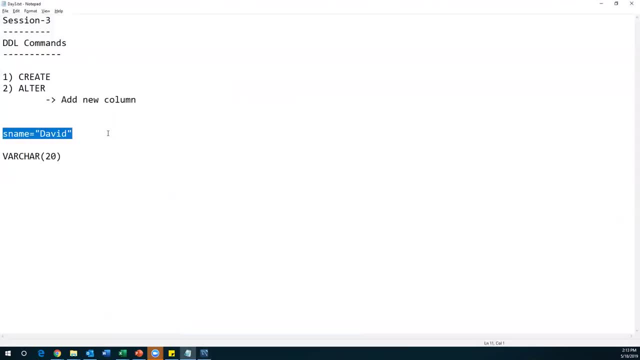 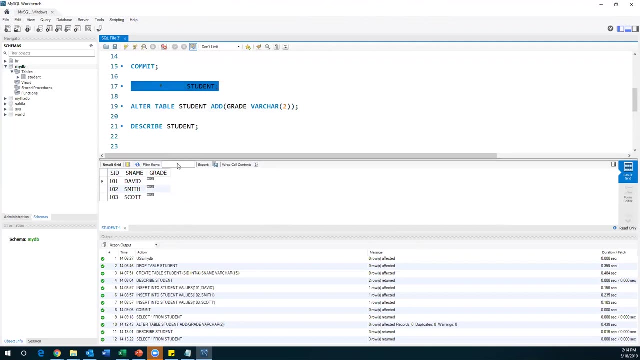 and so where SID is equal to something, so we need to write a simple query there. by upgrade update command we can add the data in the particular corner. so here we are discussing about our order command. so alter command is only works on the definition level, not the data level. okay, so now I have shown you how to add a new. 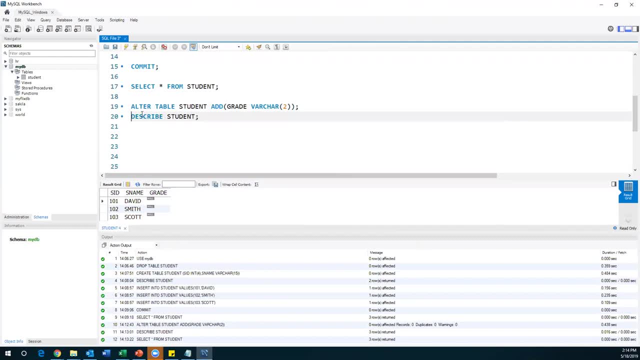 column in the table. suppose I want to drop the column. okay, I want to drop the column. how we can do that? so drop the column is I want to remove one of the column right? so to drop the column again, we have to use the same command. order order table. student orders table. 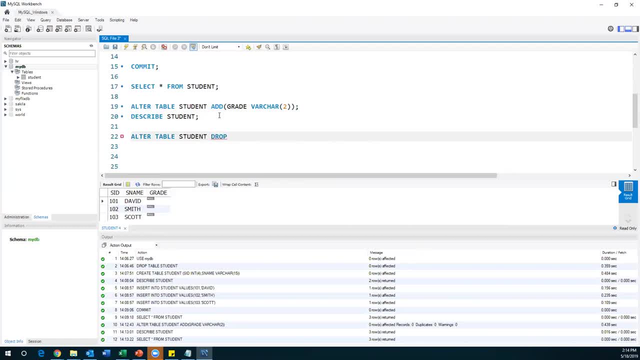 student and the command is: drop column. alter table student, drop column. and which column we need to draw? so great column is already created just now, so I am going to delete the same column. so I just remove the same bar. great, okay, alter table student and drop column grade. so this command will delete the existing column. 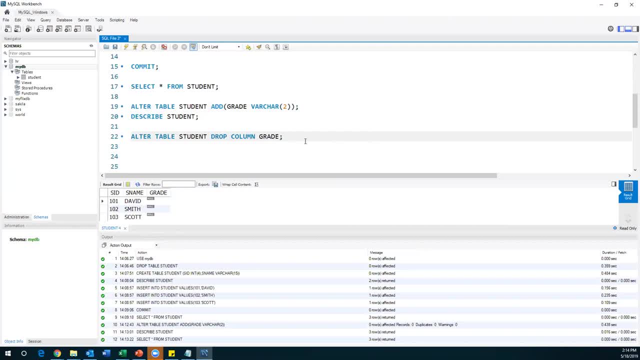 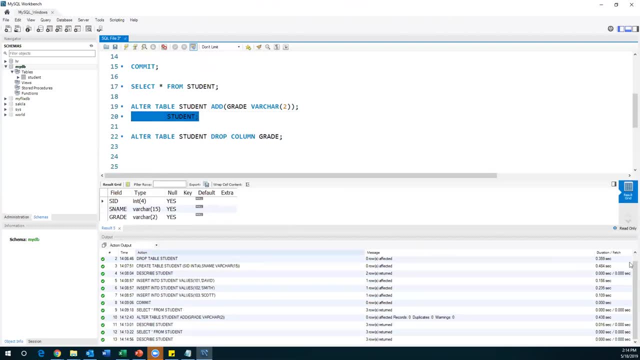 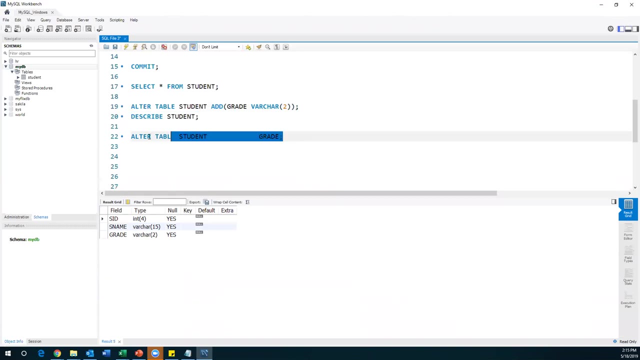 so this is also definition level command right. so when I run this code and before executing one more time, I'll show you the description of the table. so currently one second right. so currently here I have a three columns s ID s name and grade now after dropping the column. so I have dropped the column now again. 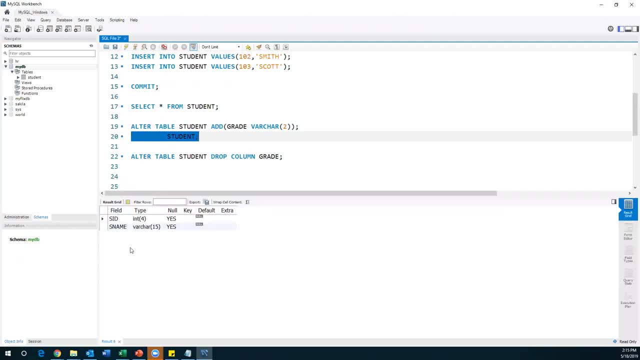 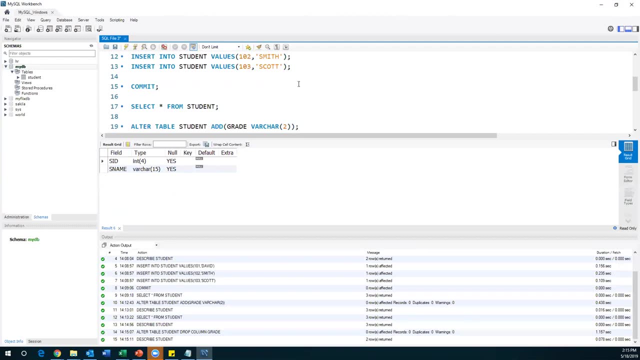 description. execute the describe command. now you can see only two, two fields here: s ID and s name. so we have dropped the particular column that is called as a grade column. okay, so this is how we need to use order command. so we have seen two important things. one is how to add a new column and how to drop. 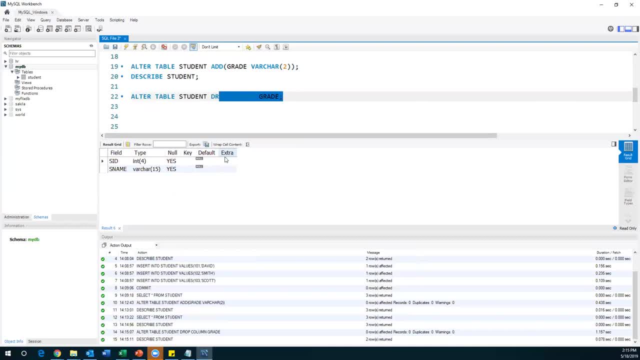 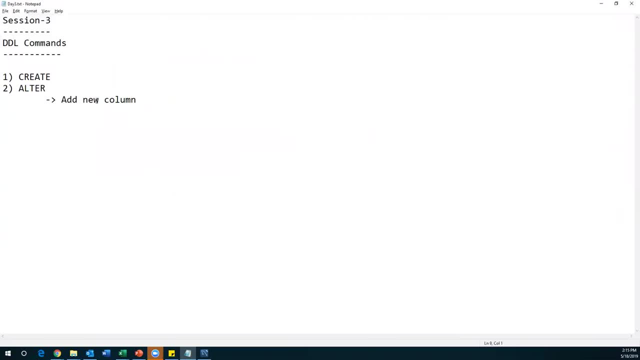 the existing column so we can also modify the existing one. so we have seen multiple operations space one is. we have seen how to add a new column and then the next operation: we have seen how to drop a column. drop a column from a table. now I'll show you how to modify the existing column. modify existing. 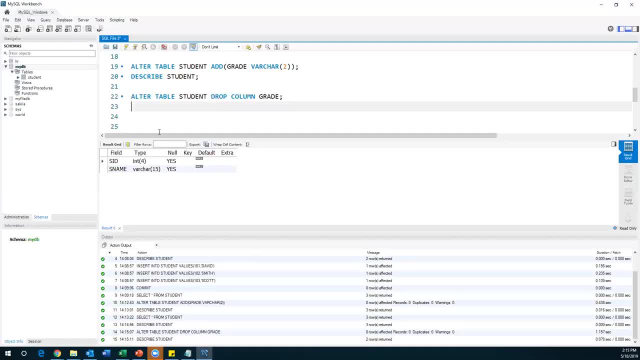 column. suppose here I already have two columns: s ID and s name. suppose, for example, here this particular table s name field allows only 15 characters of the name, so the name should have only 15 characters. below 15 characters also will be allowed, but if I want to save a, 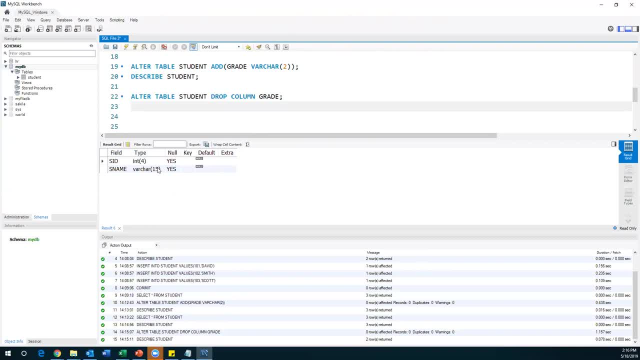 name above the 15 characters. it will not allow us. okay, it will give the error. so now what I want to do is: I have a list of names. all the names are above the 5- 15 characters. so what I should do now? I should modify this particular column so I should modify this particular column means I need to increase the size of the column. so how to increase the size of the column? so to increase the size of the column. so again we have to use a same command: alter table student, alter table student and modify. so this. 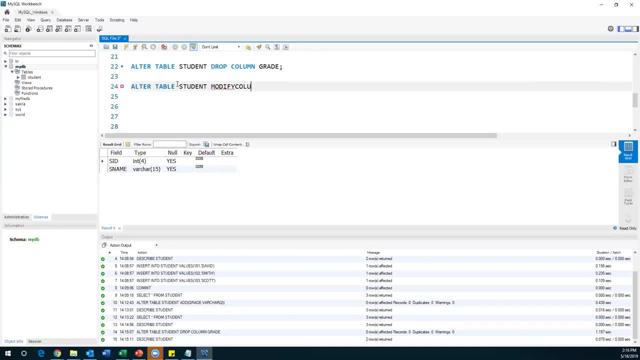 keyword you have to use alter table, student, modify column. so previously we use drop column, so this time I'm using modify column. okay, drop column is done, so modify column. and which column we need to modify? we need to specify, so s-name column. I need to modify S name and we need to also specify it to Elo. 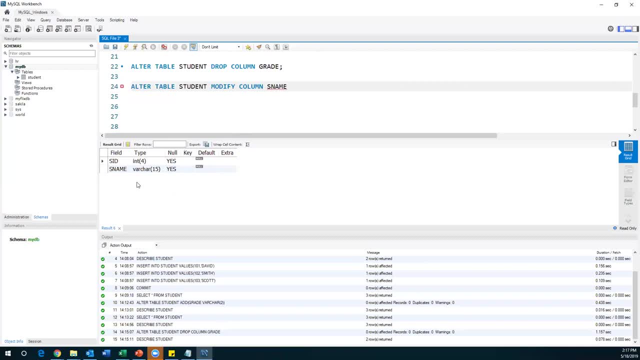 specify what is the modification we have to do. so the modification is: I want to modify the data type size. okay, previously it was 15, now I need to increase to 20, so s name where care of 20. specifying: okay, alter table student. modify column s name where car of 20. and one more important thing is suppose I already have 15 character size. size is 15 and I already have some data, which is all. all the data is the below the 15. so if you want to increase the size of the column, we can still increase it, no issues at all. but if you want to, 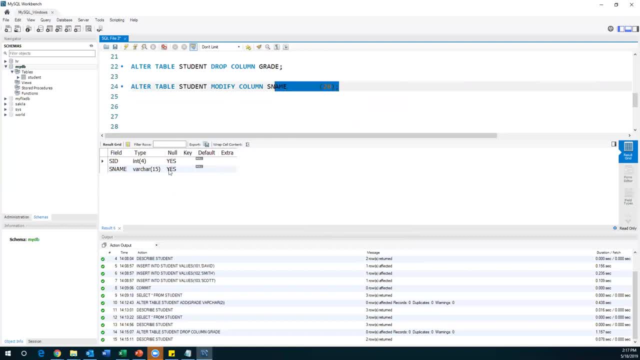 decrease the size of the column. we have to clear that particular column. we should not have any data on that particular color and then only we can decrease the size of the color because already have some data is supposed. I have some data with 15 characters. some of the names are: 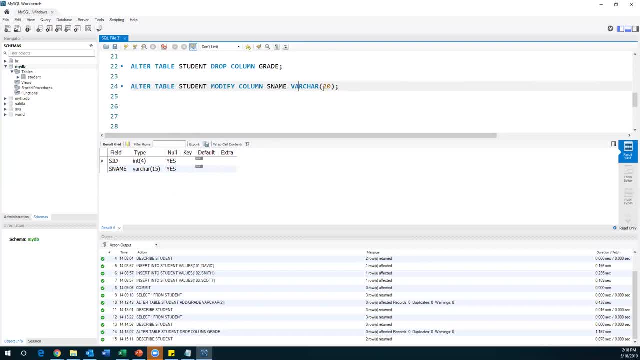 15 Po ela. these are the material data. this data is which is important. Now I'll try to reduce the column size as a 10.. So then, what happened to the records? available records? So there will be conflict, right? So before decreasing the size, we need to make sure data should be clear. 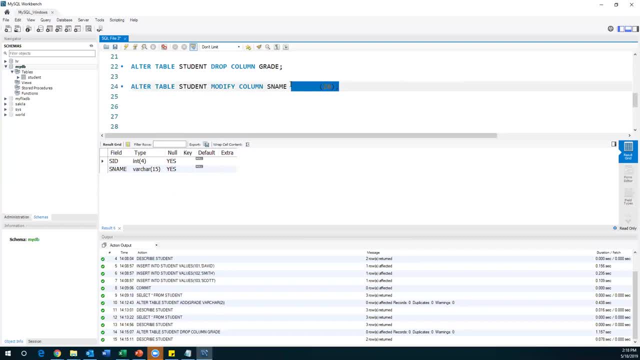 So first we need to remove the data and then we should be able to decrease the column. So that's a prerequisite for that. But to increase the column we don't have any restrictions because already, whatever data is available, it is still there and the size of the column will be increased. 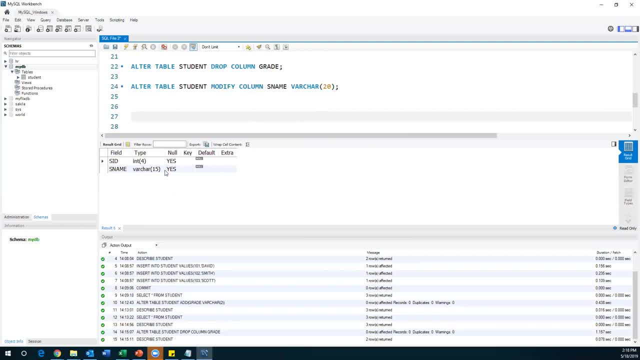 From the next round we can insert the data which is more than 15 characters. Okay, So let me so first of all, currently have bad car 15 now after executing this command. So I have executed successfully again. do the description the script: student. 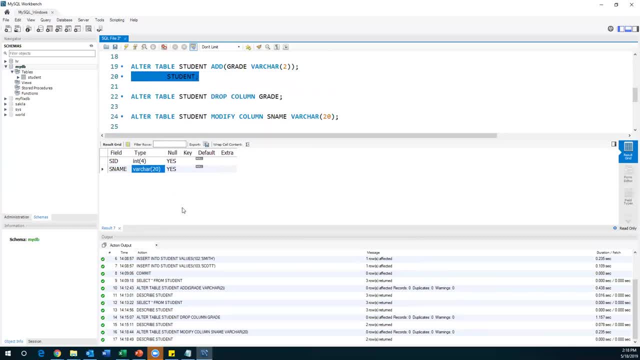 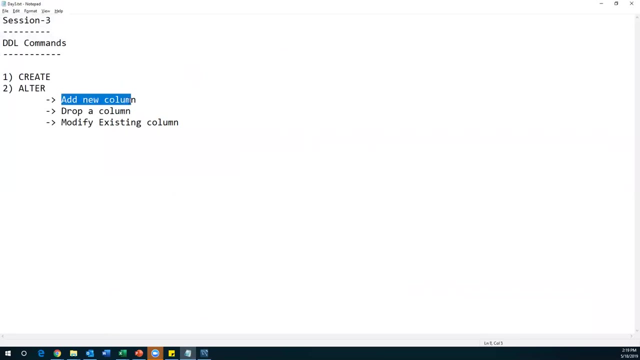 So now you can see where cat 20 has been changed. So now we can also store the data above 15 characters, again below the below 20 characters. Okay, So this is how we need to Use the alter command. So alter command will be used to add a new column into the table, drop the existing column. 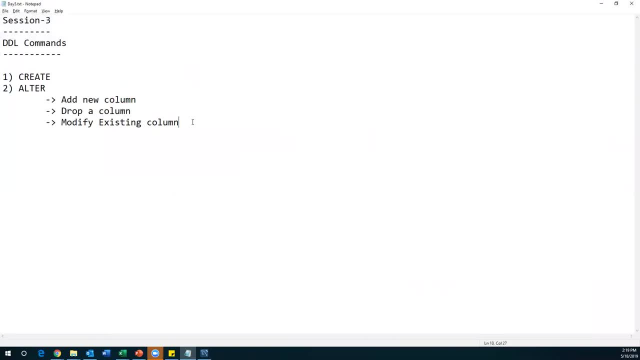 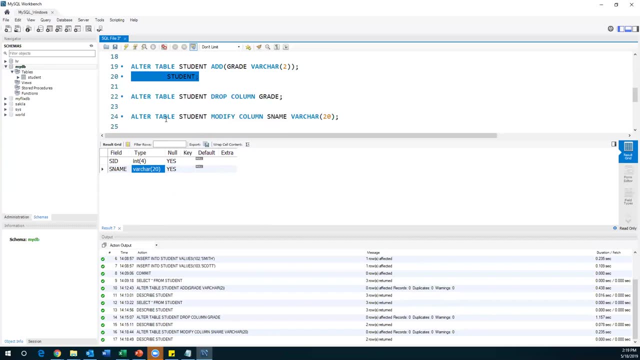 modify the existing. modify the existing column means we can increase the degrees of the site, increase or decrease the size, or we can also change the data type if you want. Suppose you're currently the uh column as name is worker And suppose I want to change the data type. 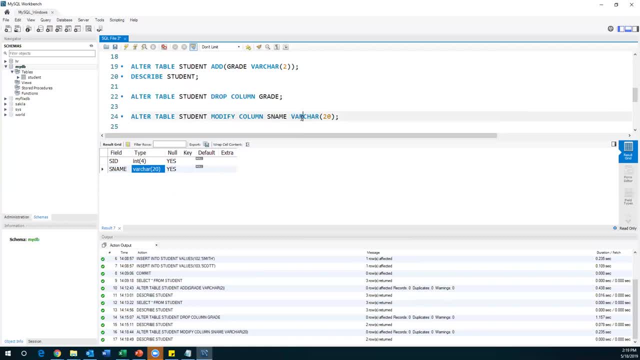 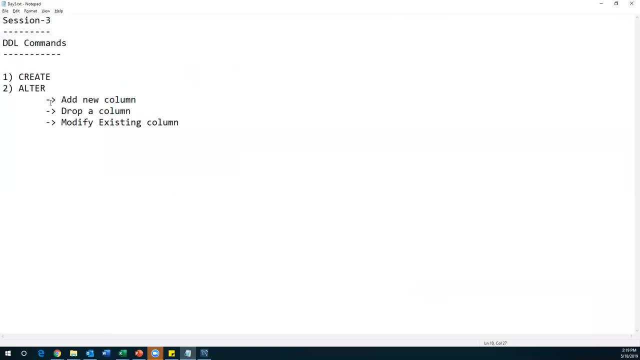 I want to use a different data type. You can also change the data type, Okay, But in that case we need to make sure, Okay, The data should not be there in the corner. Okay, So this is how we need to use alter command for adding a new column in the table, for dropping. 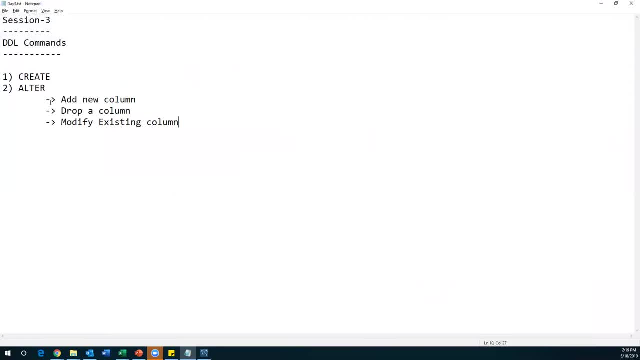 a column and modifying the existing column to increase the degrees of the sizes. And now one more thing we can do is renaming a con. So how to rename a column? So we have another command. We can still use outer command to rename the. uh, rename the columns. 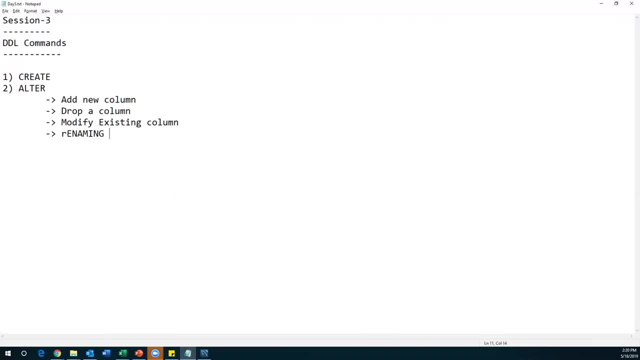 Okay, The another operation is Renaming column. So I already have some column in the database, but I want to rename that. I want to give a new name to the column, So rename, rename the column. So this is another operation we can perform by using alter command. 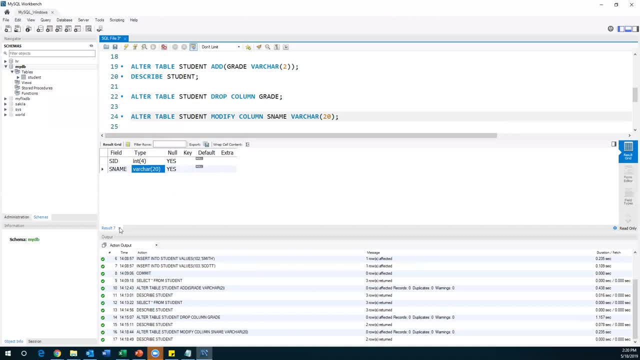 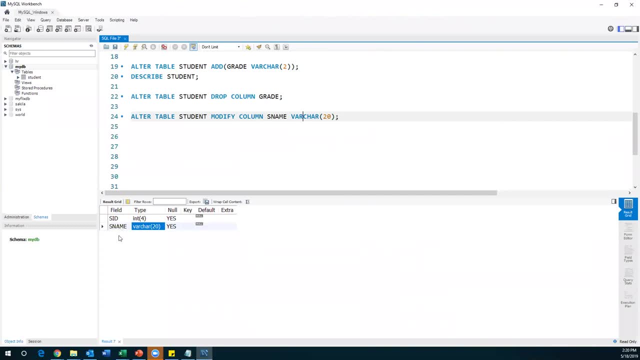 So how to rename the column in a table? So currently in my table, So currently in my table, So SID S name is there. So I want to rename these two columns So instead of SID S name is there, Okay? 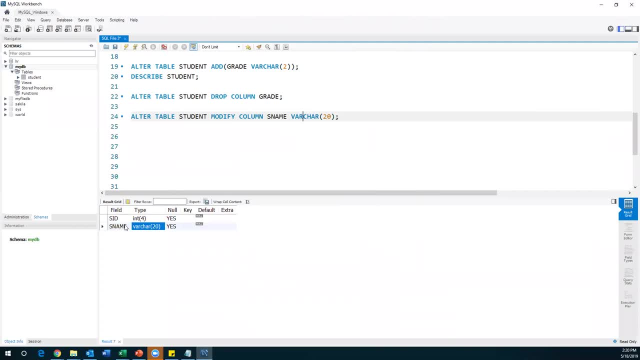 So instead of SID, I will say STU ID, instead of S name I'll say STU name. or else I can change one name and S name. instead of S name, I'll say STU name. I want to rename the column. 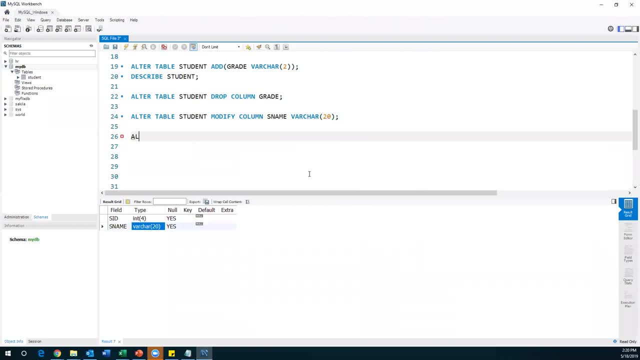 So how we can do this? again, the same command: alter, alter table, alter table student. So every time we need to specify the student, a table name, So alter table, student. And here we use another keyword called rename. So we have use alter student, drop column, alter student, modify column, alter student, rename. 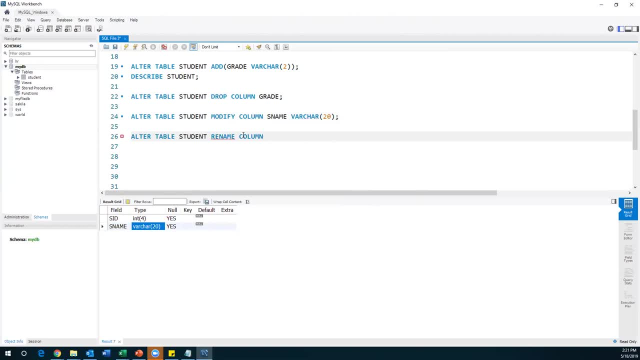 column. Okay, This is another problem: Rename column, And here we need to specify the old name and the new name. So the old name is so old name is S name, right, So the new name is S name. two: We have to change with a new name. 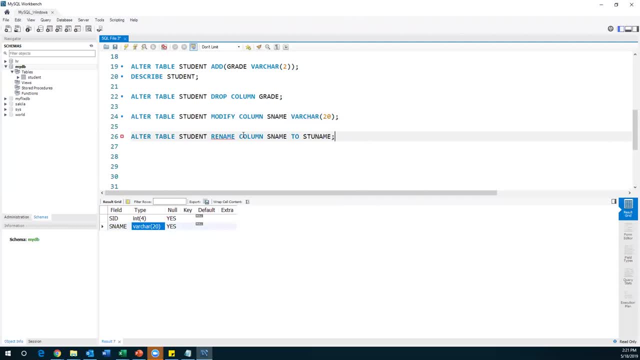 So as this STU name. So this is a whole new name. Okay, So this is a whole command. So: alter table student. alter table student. rename column S name to STU name. So S name is already there, So now I'm going to change it to STU name. 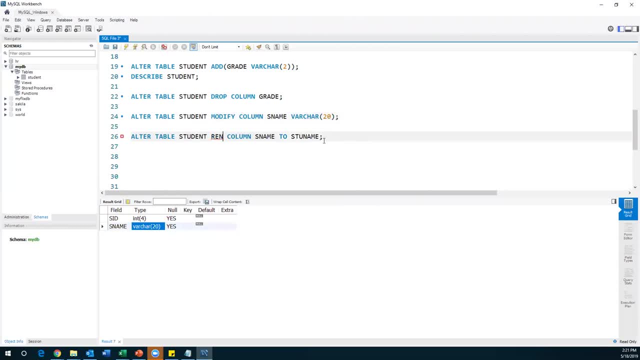 So this is how we can rename the column, And I think spelling is mistake: alter student, alter table student. uh, rename, I was giving error. Just a moment. Yes, Yes, Okay, Okay, Okay. So the problem is: yeah. 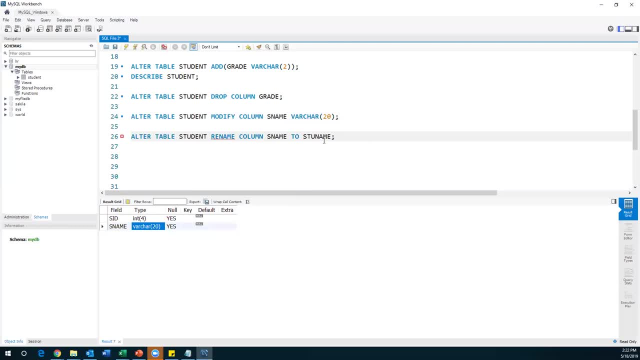 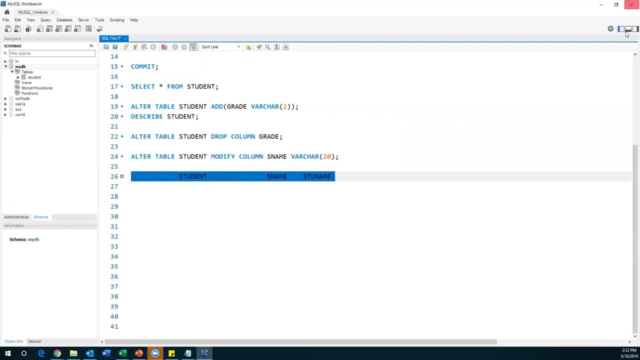 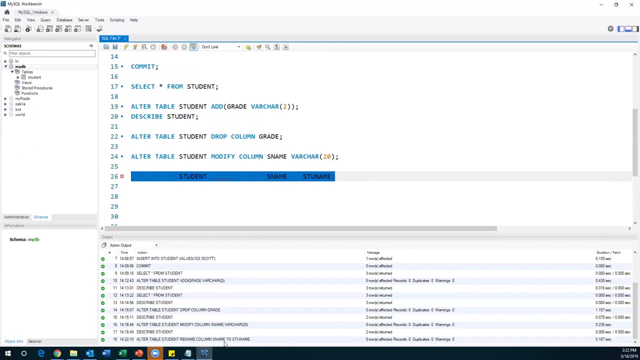 Rename is there. Rename column S name is good. Let's try this. So execute this column. Let's put this one: Okay. So I think this is a successful execute. So alter table. student rename column name S name to STU name. 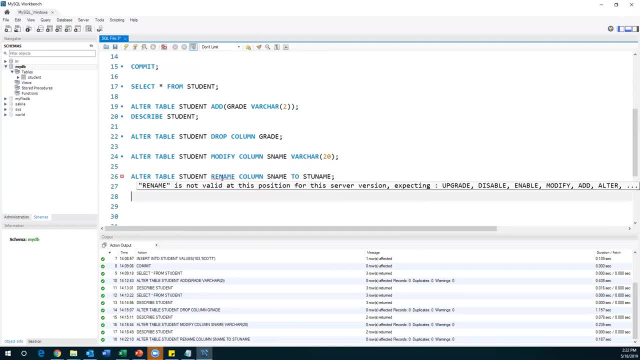 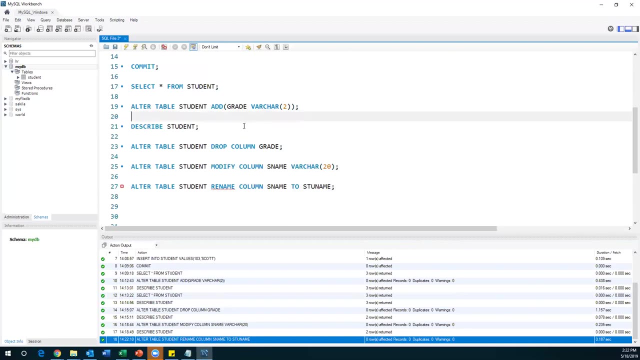 So it is giving some reason some error. Maybe this is not a supported in some version, but still fine. So I have executed this command. It is successful executed. So alter table. student Rename column s name to s name: stu name. Now I will describe the table again, So I'll execute this. describe student. 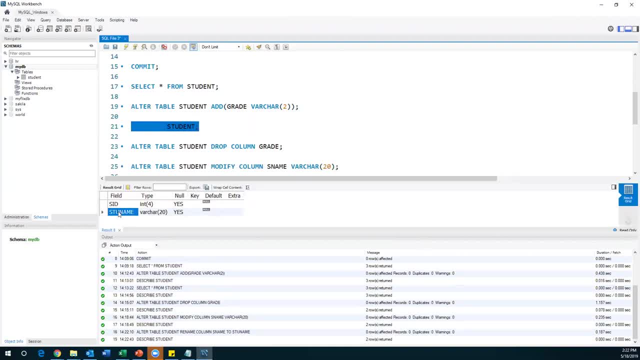 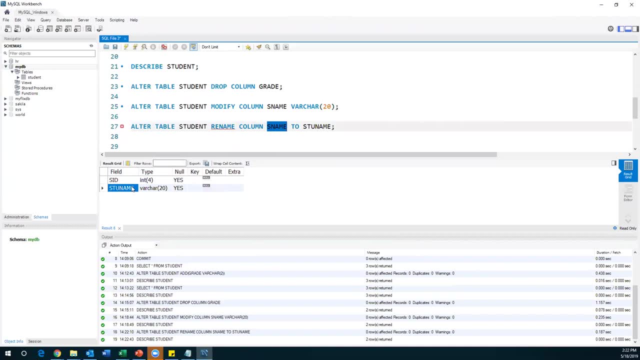 Execute this. now in the description I can see the name is changed here: Stu name, so previous it was s name, now It is a stu name. Okay, so these are our four operations we can perform using alter command so we can add a new column to the table. 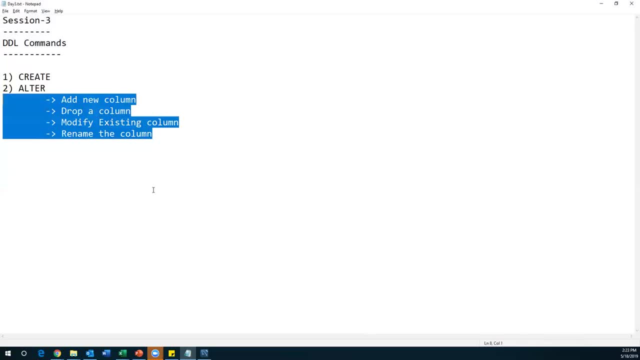 We can drop the existing column, We can modify the existing column and we can rename the column. So these are all. operations are performed at the table level. tables and columns level right. So that's the reason these commands are comes. this alter command comes under the data definition language. 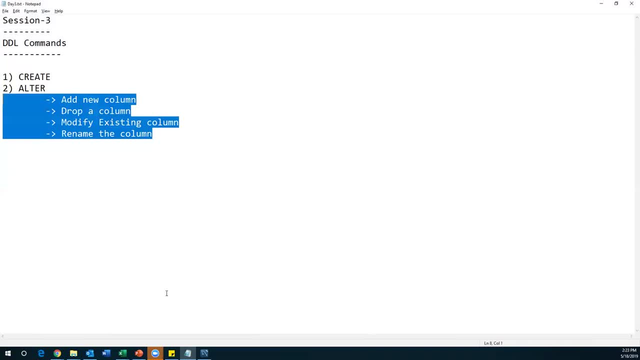 So we have seen create and order, So we have few more commands under DDL. The next command is drop. Drop is also comes under the DDL command, drop. and there is one more command called as a truncate, and Actually delete is not comes in the DDL command, but we need to also. 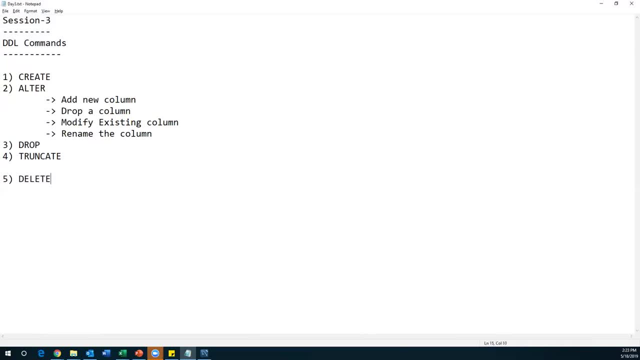 Compare these two commands with the delete command. So delete is not comes under the DDL command, delete is comes under the DML command. Okay, but drop, truncate, delete- these commands seems very similar, but there are a lot of differences, are there? So first of all, let me finish this drop and truncate, then I will discuss about the delete. Okay, so 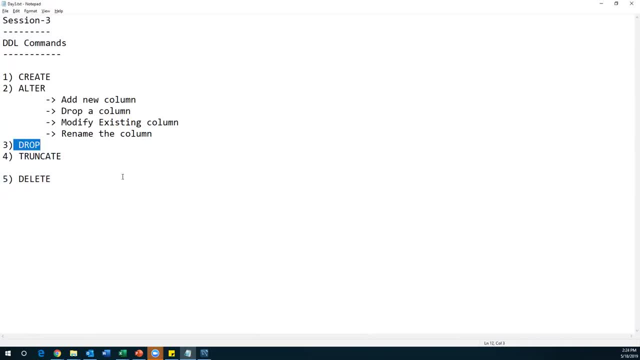 I er, I like this, okay. So Okay, Let's finish the database. Let's try to drop the database So we can see if we want to吉 to create an order. We have seen so what is drop, so drop, use it to. 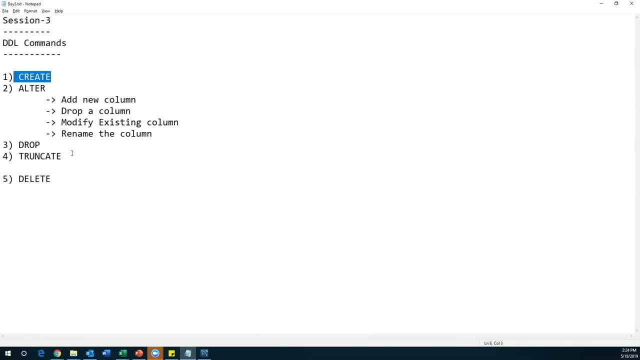 Normally drop the database object. if you want to drop the database, Or if you want to completely remove the database, just drop database. So first we need to compare these two, then we go for delete command. So in the DDL we have a drop command. 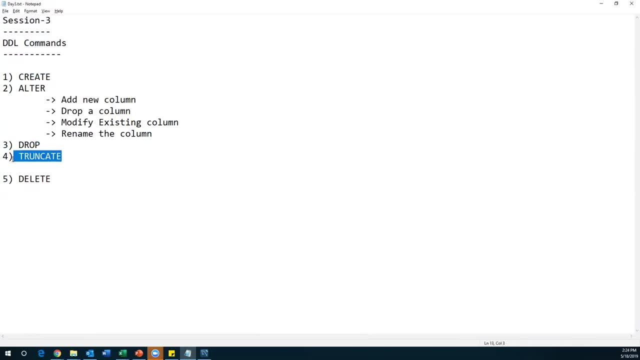 and we have a truncate command. What is the difference between drop and truncate? So drop command will completely drop the table definition, Data, columns, definition, everything is gone. So completely table itself is gone. But when you use truncate command, table's still present, but the data will be deleted. 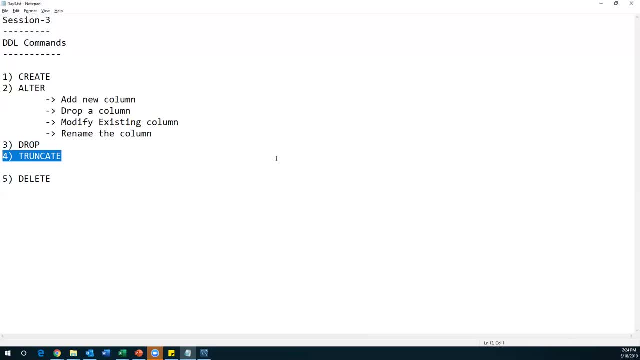 So table structure's still present, but only the data will be deleted. So when you use truncate command But we have another DML command, delete command. When I use this command, this will this one and truncate will work similar way, but there is again difference, is there? 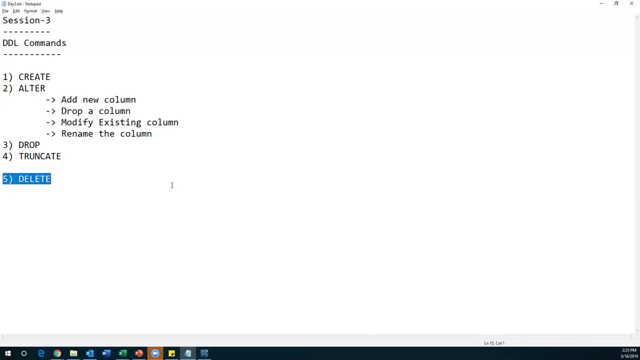 So when I use delete command it will also remove the only data. It will also remove only the data from the table, but still table is present. Even when you use a truncate command, here also the data will be deleted, but still table structure is there. 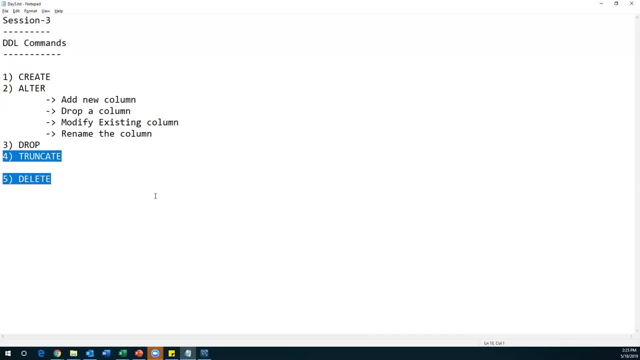 And truncate delete will seems very similar, but what is the major difference between these two are, if you do truncate, the data will be permanently removed from the table. We cannot roll back the data, But when I use delete command, the data will be removed temporarily. 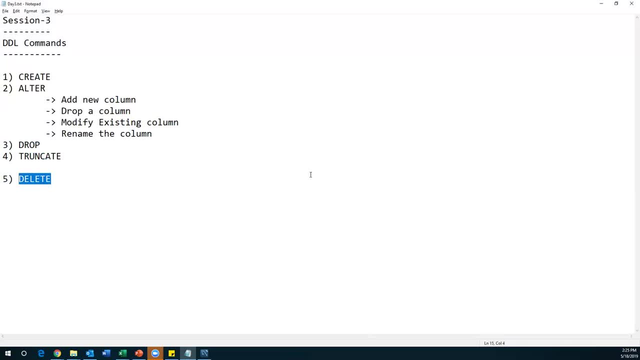 Even though if you remove the data, even though if you deleted the data, you can get back the data, You can roll back the data. So that is possibility we have in the delete command. So drop is a drop and truncate- These two are comes under the DDL command. 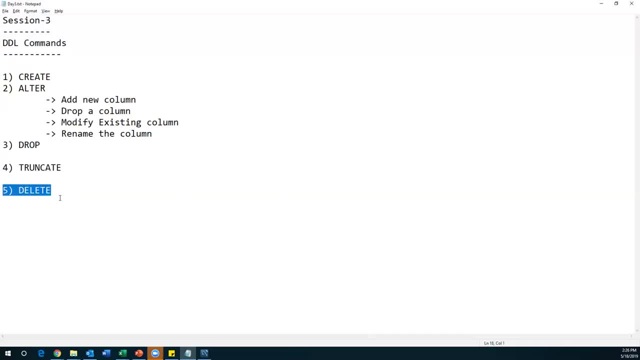 So delete command comes under the DML command, because this command works only on the data, not the table level definitions. But what is the exactly difference is drop command will completely drop the table, Data structure, table definition. everything will go on permanently. 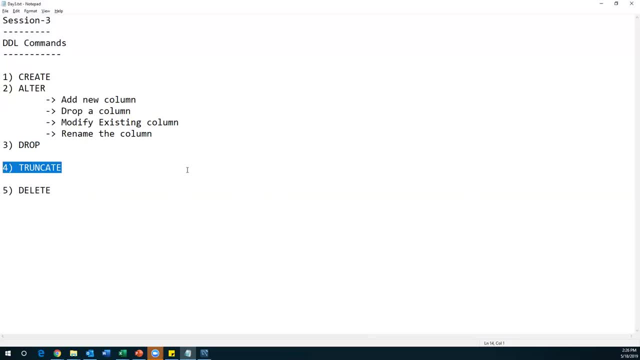 And truncate command will also delete the table data, but table still present. The table structure is still present, but data is removed permanently. And delete also removes the data from the table Still. table 2, structure is present, but the data can be rolled back. we can also get back the. 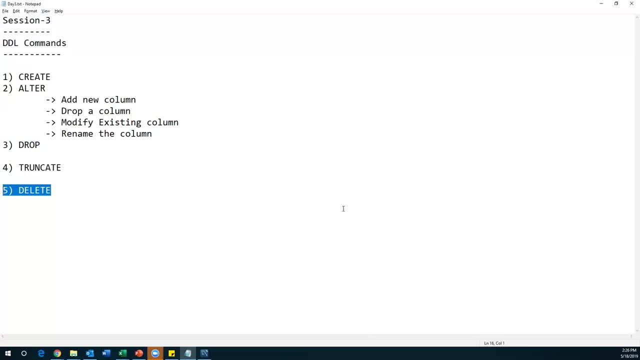 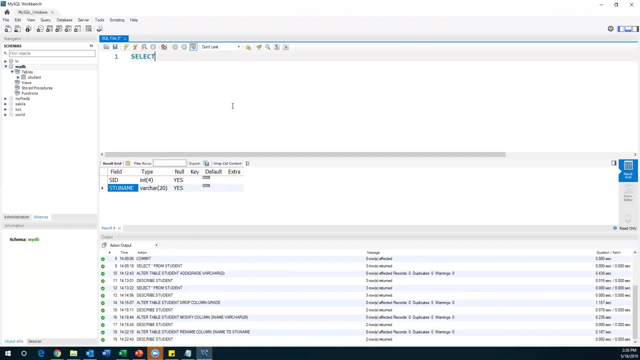 data from the delete. so these are the basic differences between drop, truncate and delete commands. okay, so now I'll show you practically how we can use this commands. so go to your workbench. so I'm just removing this command. so currently I have a table right, so select a star from student. so I have this particular. 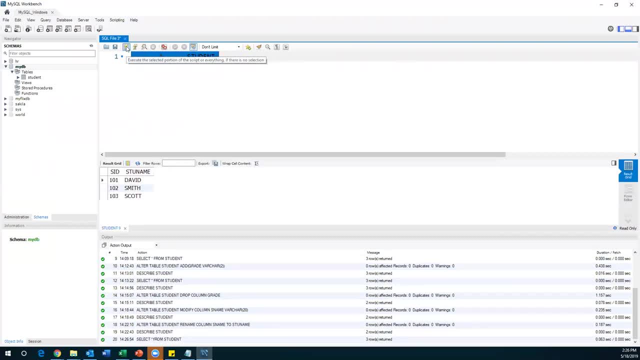 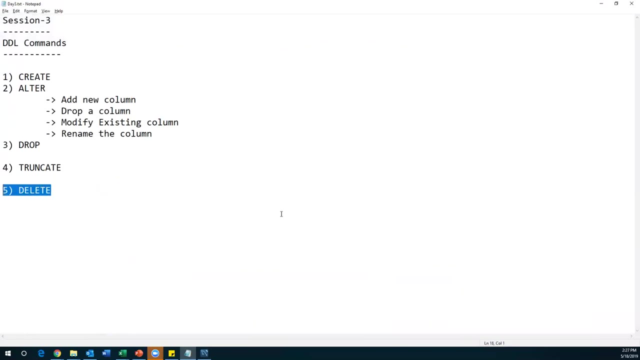 table. when I execute this, you will get some data right. so now what I want to do is the first thing, I will show you delete, truncate and drop. so I will first to show you delete command, and then I will show you truncate command and then, finally, I will show you drop command. okay, so first I will show you delete. 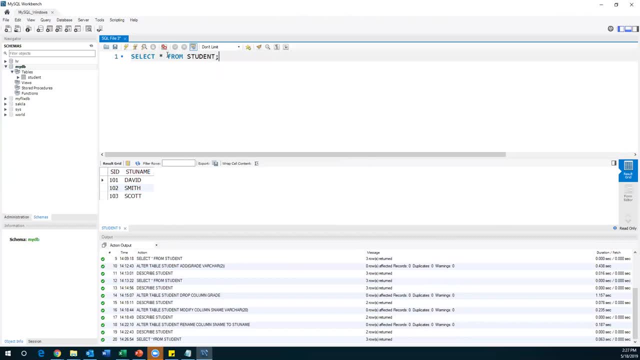 command how to delete the data from this table, and I will also show you how to roll back the data. we can also roll back the data. okay, so now, before you go to your workbench, you have to go to your workbench and then you have to. 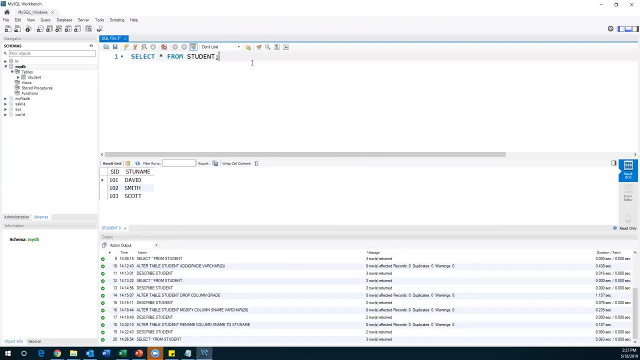 that what we need to do is we need to exude a command for less set autocommit zero only in the MySQL. this power, this option is available. so what is autocommit means? so we need to understand this guy's. what is autocommivity? in my sequel, whenever you do set in action on the table, like you. 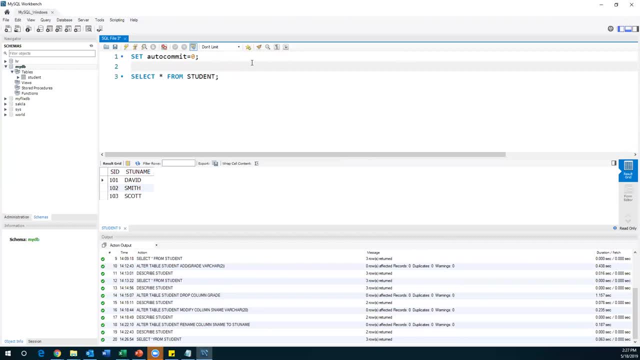 have inserted to some data, or you have updated the data or you have it deleted, that it so, as soon as you have done, set in action, my MySQL by default commit those records in the table. commit in the sense It will make permanent action. That is a comment. So whenever you do set an action or whenever you execute your DML action, 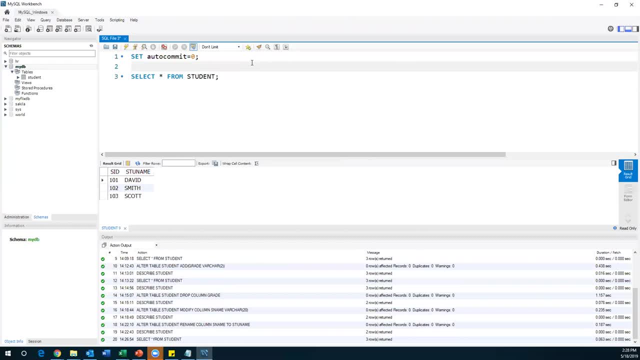 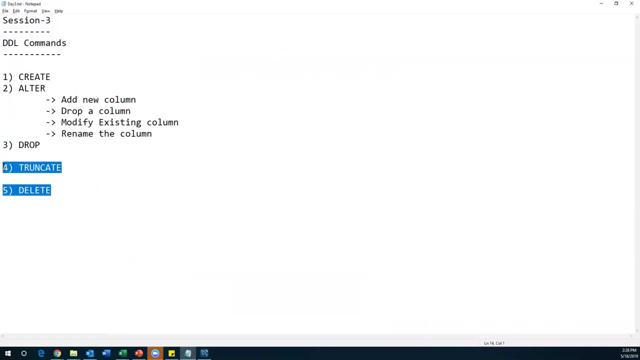 Either it can be insert, update or delete. my sequel by default commit those transactions in the table by default, So in that particular context. so these commands will behave differently. So truncate command, delete command will behave drink differently because auto committees enable so, to Enable these functionality like drop, truncate and delete or if you want to get back the data. 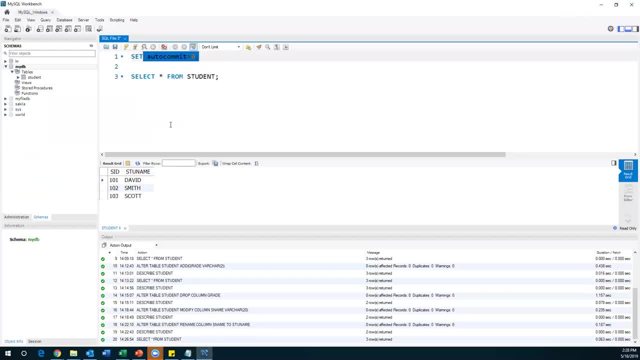 We need to make this property become zero. set out of committee, We should make it as a zero, So then it will not perform any automatic parameter. So auto commit is a one of the property- my sequel- because of this, auto commit feature is enabled, So by default this value is one. auto commit value will be the one. 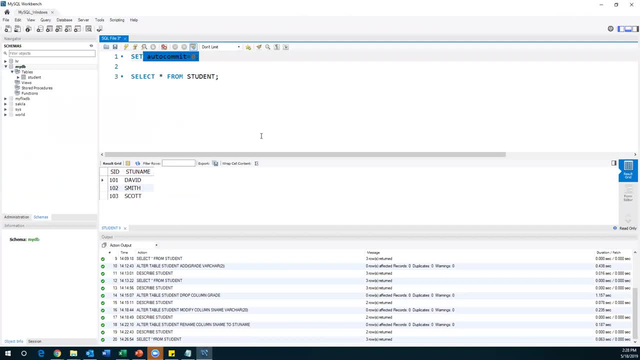 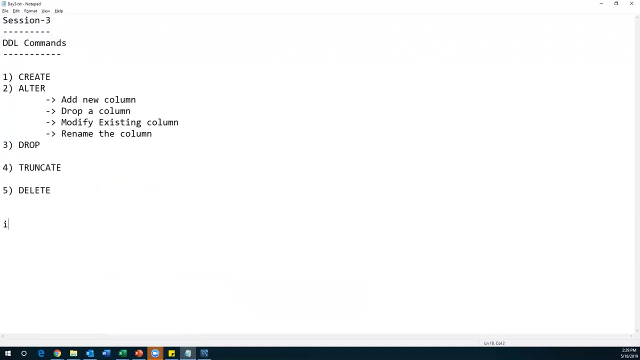 So when auto commit value is the one, so automatically whenever you do set and transactions permanently saved in the database tables. Ok, so this is a scenario guess. Let me repeat once again, Suppose I have inserting some data. So exactly, we need to understand what is out of comment, this important feature of my sequel, and we don't have that particular feature in. 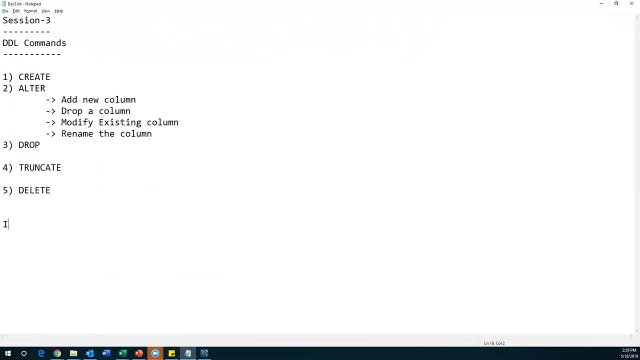 any other databases. so here, While inserting some data, right, So some inserting data. let's say, I have inserted some data, I have inserted some data in the table, in the table as soon as I have inserted data, so the data will not be stored in the table. 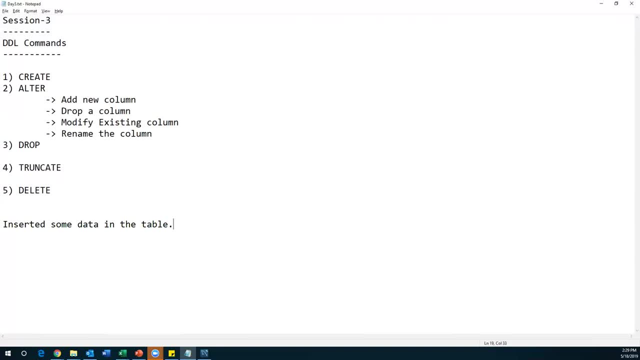 permanently. okay, the data will not be stored in the table permanently. after insertion is done immediately you disconnect to the disconnect from the database and again reconnect and see the table. you don't find the data because insert, update, delete commands will not perform the permanent actions. it will. 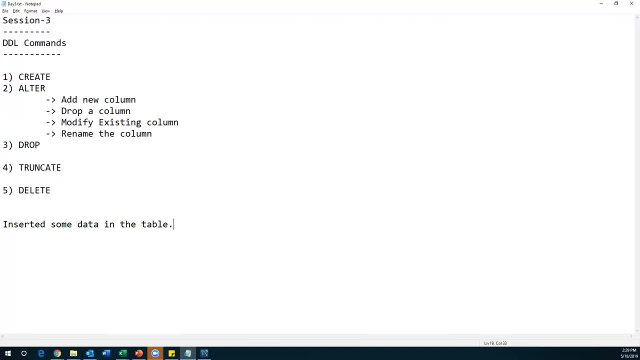 just insert the data table or update the data and modify the data. okay, delete the data. so after doing these accurate actions, we need to perform the commit action. so immediately we have to perform the commit action. so what the commit action means? whatever transaction we have done, we have done like insert. 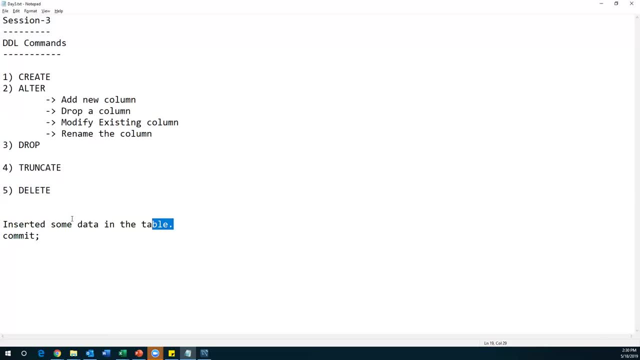 update, delete. when I perform a commit action, then these particular transaction will be permanently affected in the database. so as soon as we have executed insert command or update command or delete command, we must execute commit command to make the permanent changes in the database. okay, that's a normal way of doing, but in my sequel we no need to. 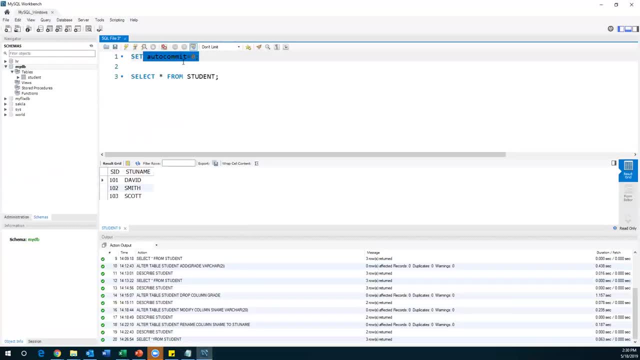 execute this command every time. why? because this auto commit will be enabled in the. my sequel auto commit is, by default is enabled. so as soon as you have done insert, update, delete, by default the data will be stored in the tables permanently- permanently. okay, so that's how auto commit works. so to use this particular features, we need to 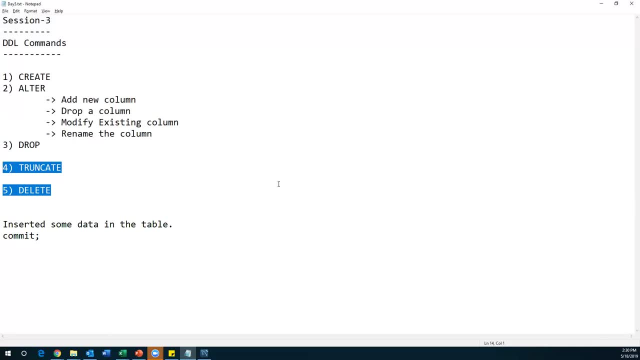 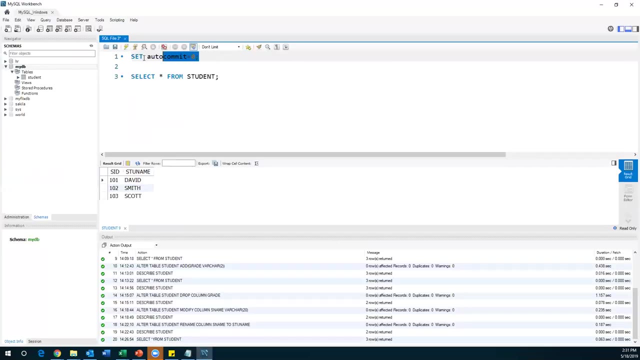 make that auto commit feature is zero. we should disable that. okay, so now what happens if I disable that as soon as I have done the insert? it will not make the permanent changes until unless we have execute this command. okay, so that facilities. we should enable that. so now I make this set: auto commit is equal to. 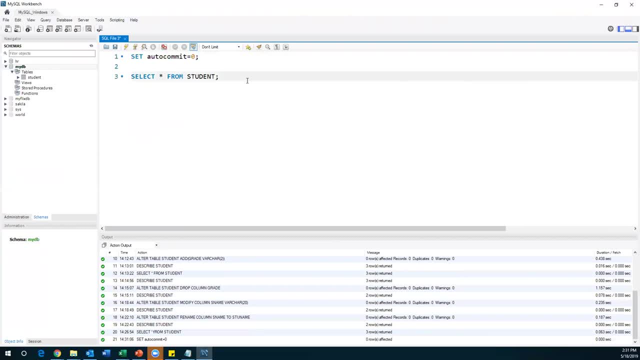 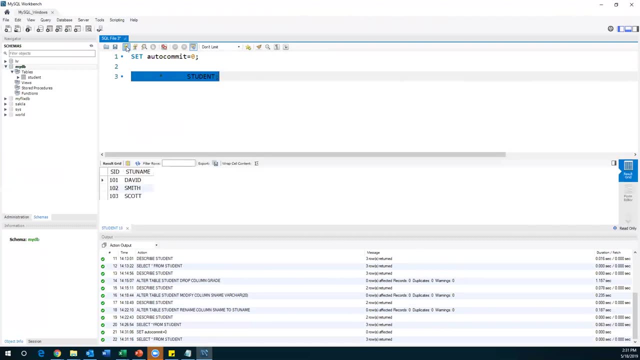 zero. now what I will do is observe guys very poor, very, very important region. so now I'm using drop command. so currently I have some data in this table, so I have three records in the table. so now I am deleting the data by using delete command and deleting the data. so let's see how to delete the data. so the 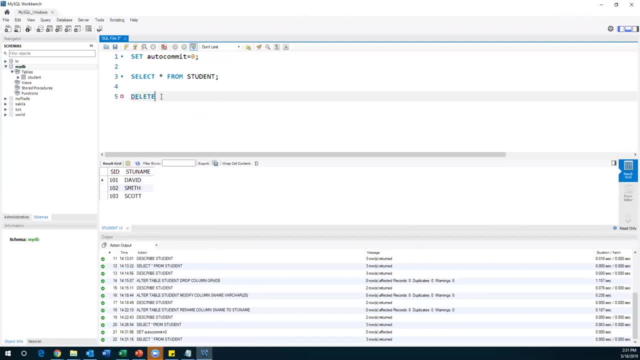 command is delete. delete from table is student, delete from student. so type: delete from table. piece. still, and now what I will do is to point that, so I'll change this expression so I have. It was a present logo, so the command is raise to zero. so now I'm gonna enter up. 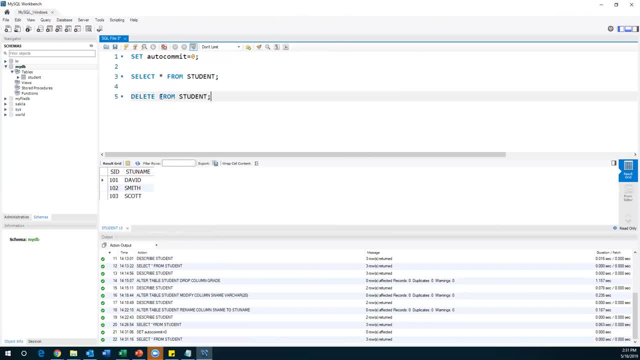 and then up and deleteValue. and now what I have? two photos. I'll change from top to bottom. So this command will delete all the data from the student. Okay, so observe this, guys. I'm just deleting the data from the student deleted from student executed. so now 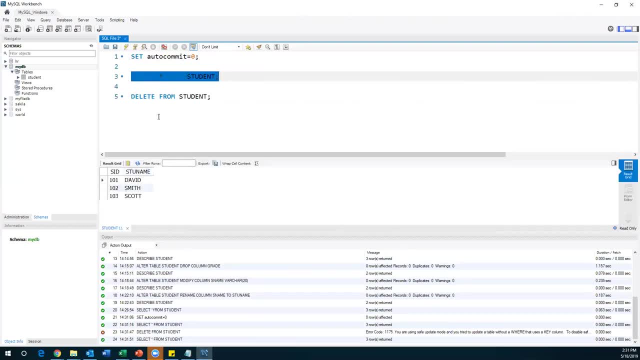 Exeggute this command. So there there is one second. It's still. there is some data right, So we have to delete this properly. So delete from student. I'm executing so because the command is not properly executed. So you are using safe update mode and you try to update a table without where that uses key color. 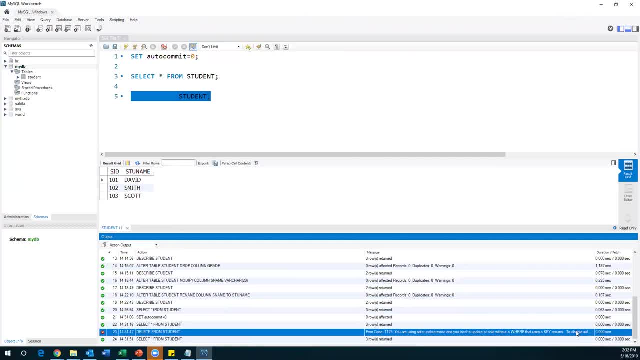 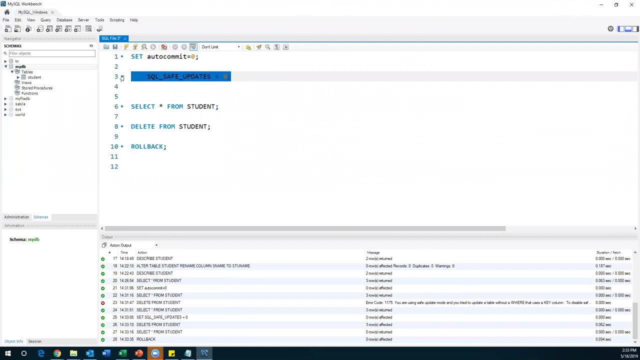 Okay. So here we need to do some changes, that we need to apply the safe mode, We need to enable the safe mode. So just a moment, I will just update that property, Sorry guys. So first time what I have done is I have just added this form: set SQL safe updates. because whenever we do deletes or updates, 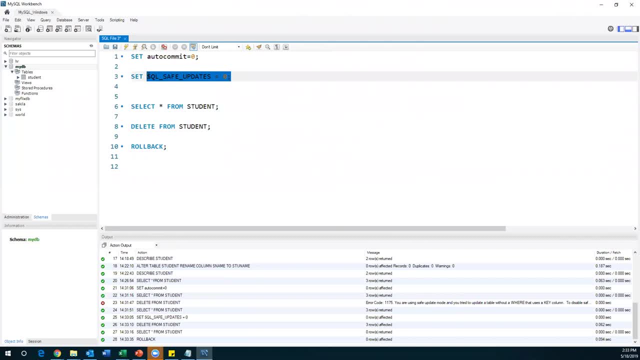 We need to execute this command? We need to set this property as a zero, then only it will allow us to update the table. So why we need to execute this one? because the table will allow us to update the table, insert the data into the table. So once I add this property, then I have deleted the data from the student. 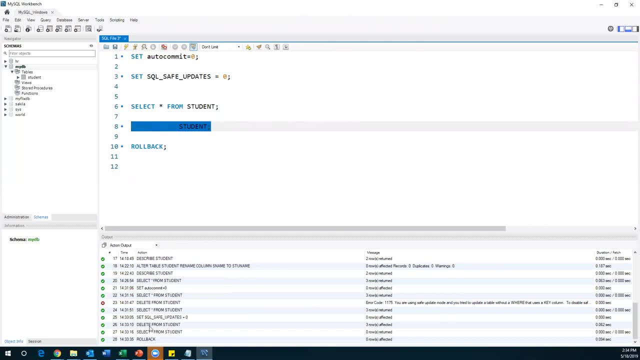 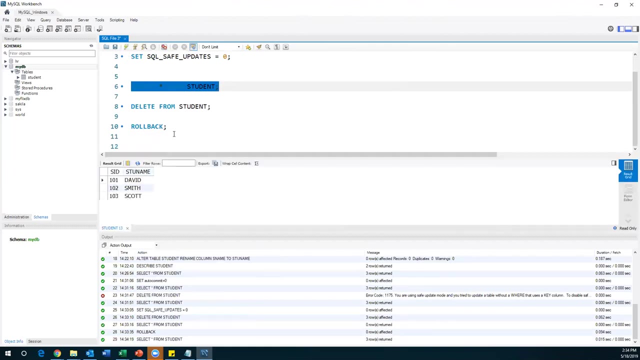 So my query is successful, so the star here delete from student. the query is successful, Then I have again executed select star from student. So now we don't have any records in the select star from student I have executed. So again I got get back the records because rollback is already executed. 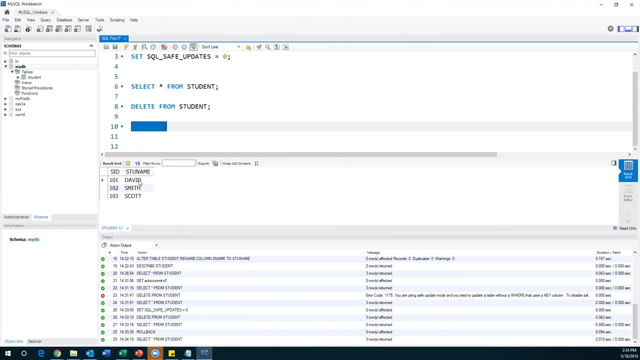 Let me show you a new data set. Okay, so one more time I'll show you so. currently I have records here and I'm deleting the data from the student and Again select this one. So currently we don't have any data now, once you executed your rollback command. 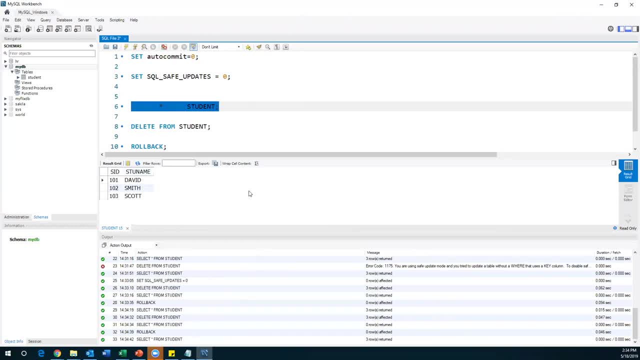 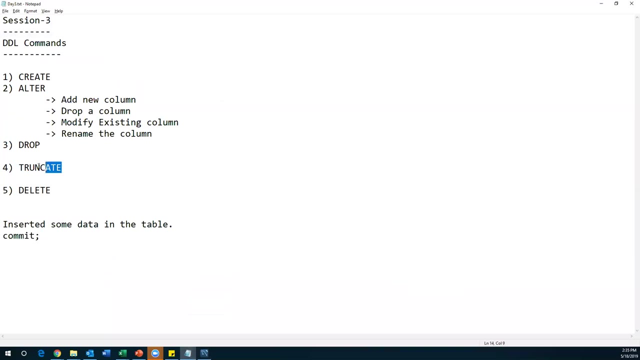 and again select the data and Then you've got the data. Okay, So what we have understood here is: Whenever you delete the data and There is a chance to get back the data by using rollback command- a facility which is provided only for delete command- but when you go for truncate command, 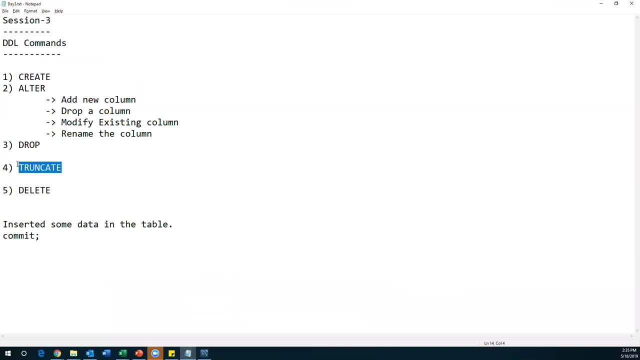 we cannot get back the data. so truncate is permanent. truncate will perform the permit action. okay. so even if you execute, the rollback command will not work. so rollback is associated with the dml commands, so like insert, delete, update. whenever use these commands, rollback works, but for truncate. 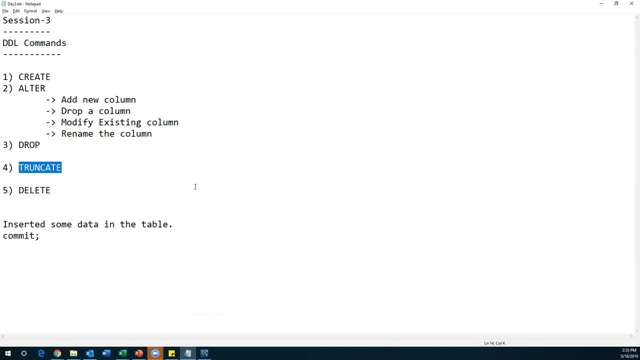 is a definition level command, data definition level command, so we cannot roll back the data. so now we have understood what is delete. so delete command will delete the rows from a table temporarily and if you want to get back the data, we just use the rollback command so you can get. 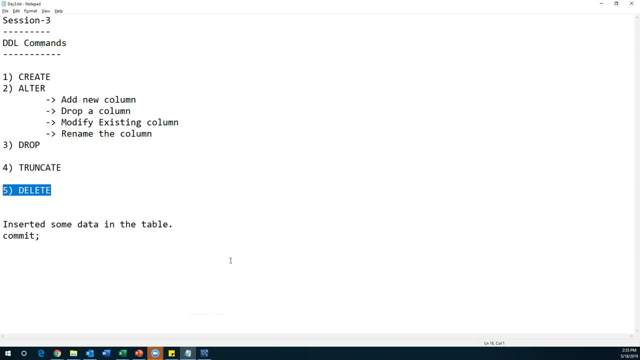 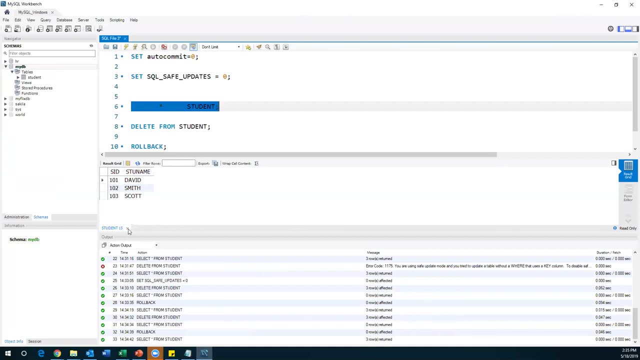 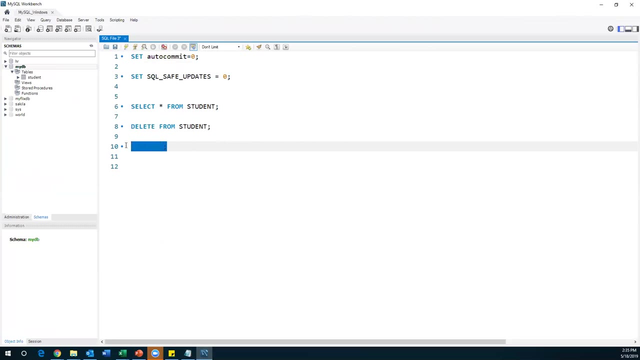 back the data by using rollback command. okay, so now suppose i'll do one more thing, guys, here i'll show one more thing. suppose here i am deleting the data. suppose i have deleted the data now when i use role back command. so currently i'm executing this query again. so there is no data and after 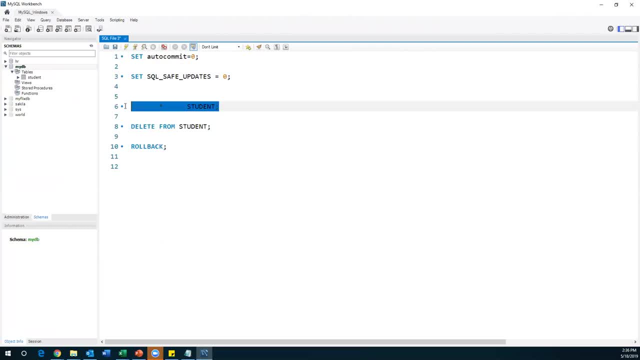 executing this rollback command. again, if i select this command- select star from student- we are getting the data right. so what i want to do is: i want to make this data permanently stored in the database. what i should do now: even i perform the rollback, i should not get the data. so i want. 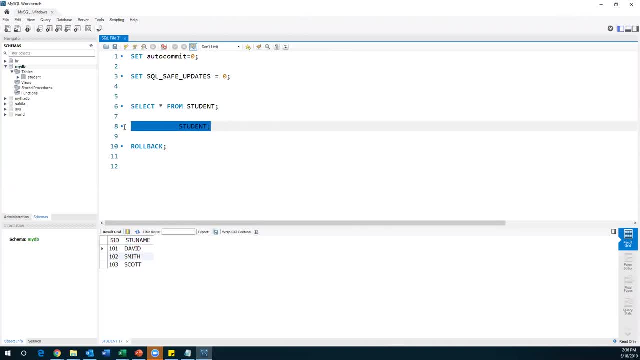 to store this data permanently. so whatever transaction delete is one of the transaction as soon as i have delete this command. this command is not deleted data permanently. that's the reason we are able to get back the data by using rollback command now, even though if I rollback command, I should not get back the data. how we can make the. 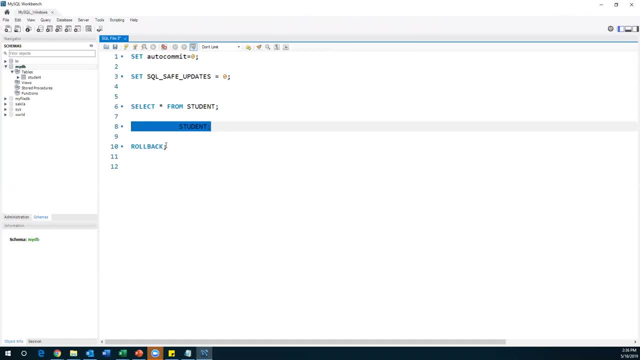 transaction permanently. so as soon as I have executed this, when I use rollback command, you are getting the data here so I can execute this. you are getting the data here. but I don't want to get like this. whenever I execute my delete command, I want to perform this change permanently affected in the database. so 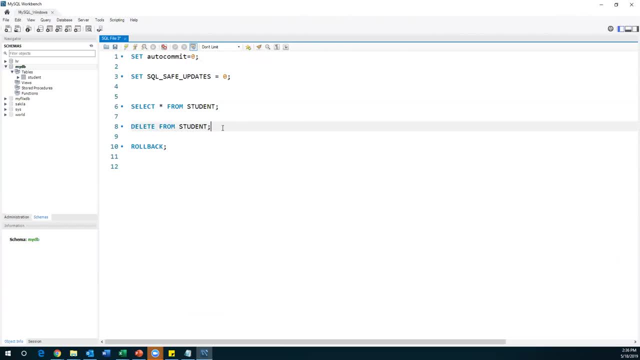 immediately after executing this command, you have to use a commit command here. come in so this particular command. once you have executed, then even though, if you see, but this particular table, I don't have a record, even though if you execute your rollback command, you will not get the data I have executed rollback. 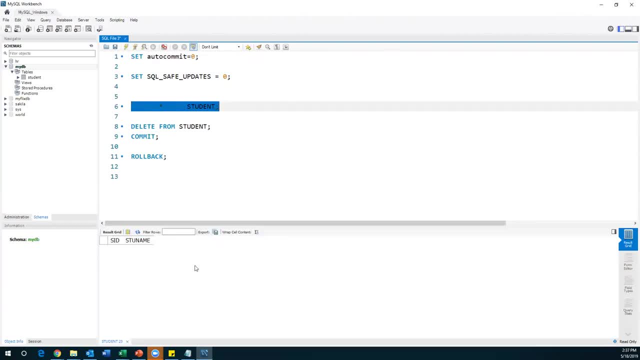 still see the table. still, you have don't have the data here, because commit is a command which will commit the records permanently in the table. it commit the changes. basically, it can be delete or update or insert whatever. as soon as we've executed your statement, commit command will commit the changes in the database permanently. we 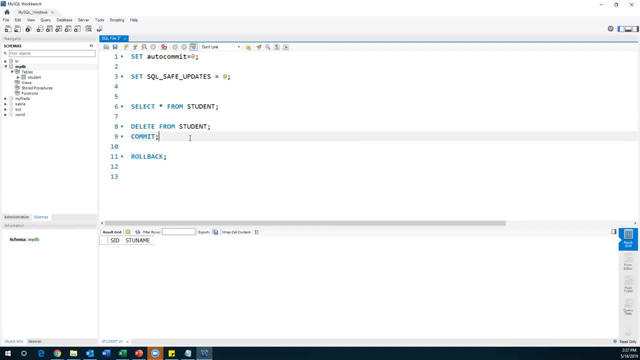 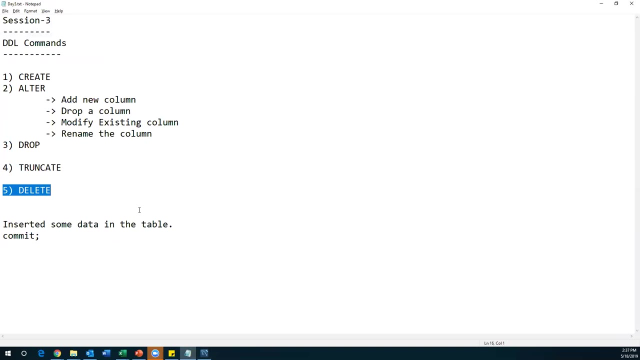 cannot roll back the transactions, but if I don't commit this one, then this particular command- is a delete or insert or update- will do changes temporarily. then we can get back the data by using the rollback command. okay, so this is how we need to use a delete command. is so now we'll go for truncate command. 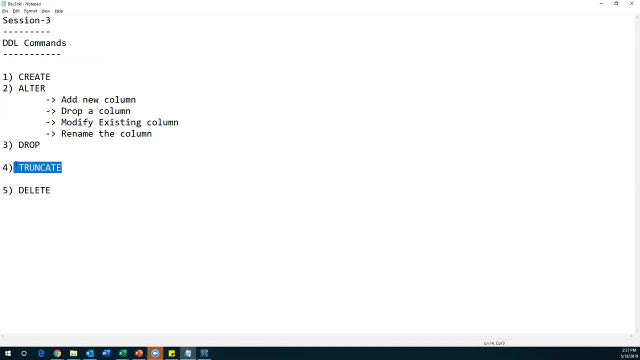 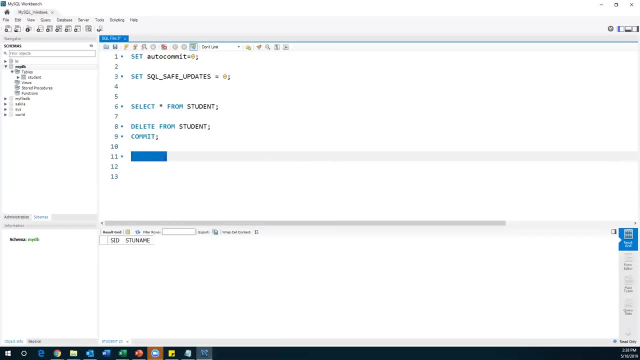 so, as I said, truncate command will again the remove the data from the table, but that is a directly permanent action. we cannot get back any data. so now I'm using truncate command. I'll show you how to use truncate command here. so the truncate command will be used like this the command is so. currently I have a. 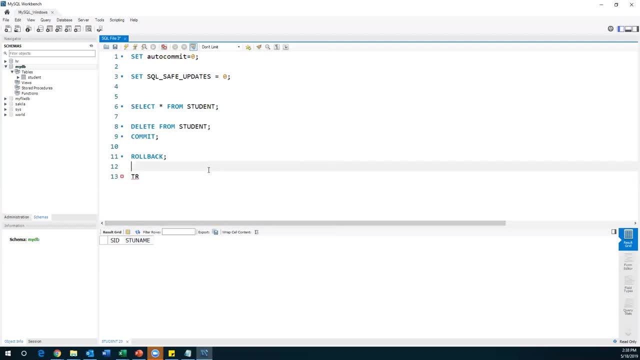 table, but it doesn't have any data right. so I will populate some data in the table and then I will use truncate command. okay, so I will use insert command, insert into which what is a table. table is student and values. here I'll say 101 and I'll say Smith is a name. similarly, I 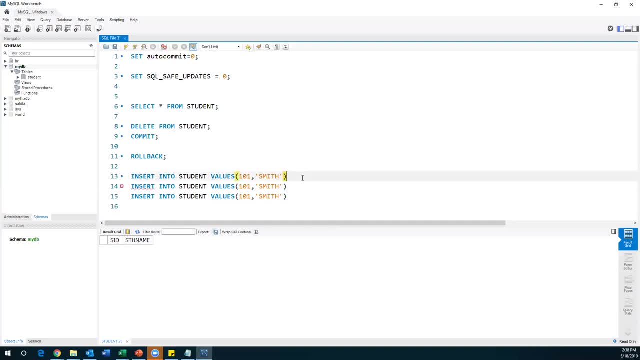 will also insert a few more records. the first record, second record, third record is 101, this 102, this is 103. so now I'm executing this data, I'll say David and here I'll say Scott. so now I'm executing these commands and it will insert the data in. 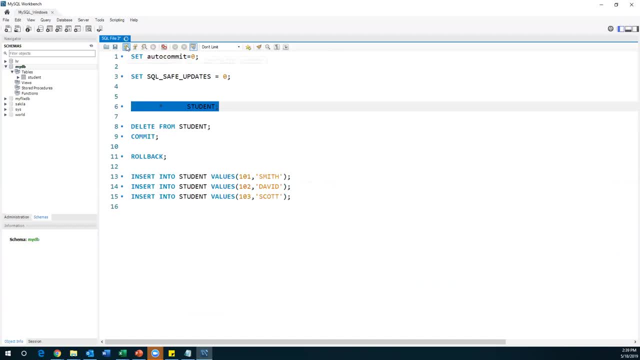 the student table. so now execute this command. you will get the data so as soon as I inserted. so please use a commit command here. okay, so then only the data will be permanently stored in the table. suppose if you enable this particular property, auto commit is on. okay, then you no need to give this command. so as soon. 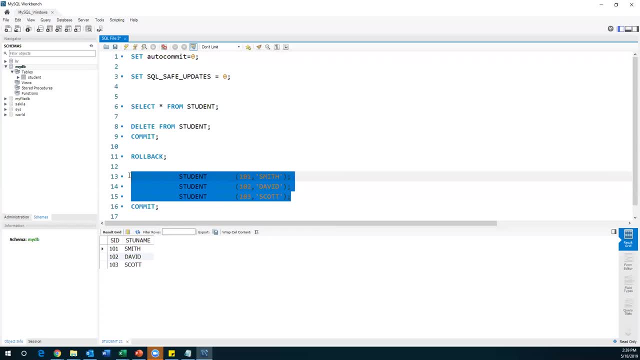 as we have executed this command by default. commit works internally, but here I have disabled this property by adding zero value. that's the reason I need to explicitly give the commit command, otherwise not required. okay, so these are connection right. these two things are having connection ways, if you. 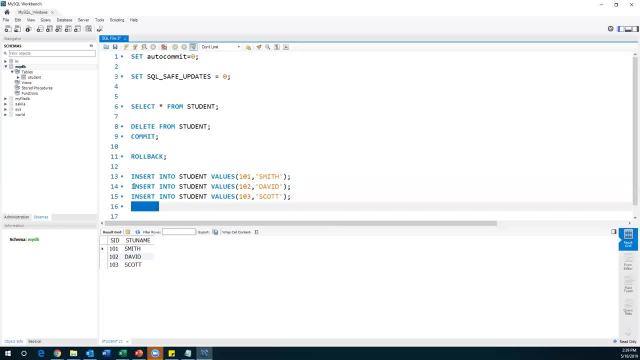 specify this property as a zero, then you must commit after completion of the transactions: insert or update or delete. whenever you do these three commands, commit must be done, otherwise the transaction will not be affected in the database permanently. and if you set this property as one, then the commit is not at all required. so by default, as soon as we have, 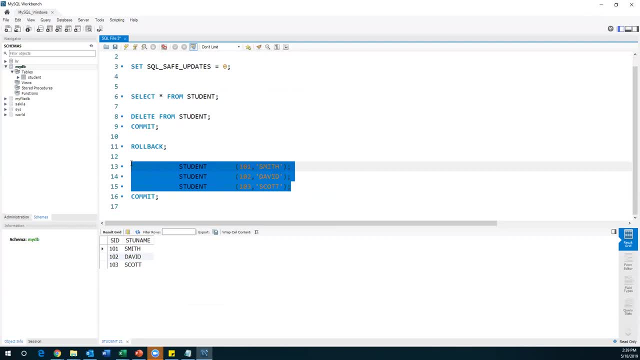 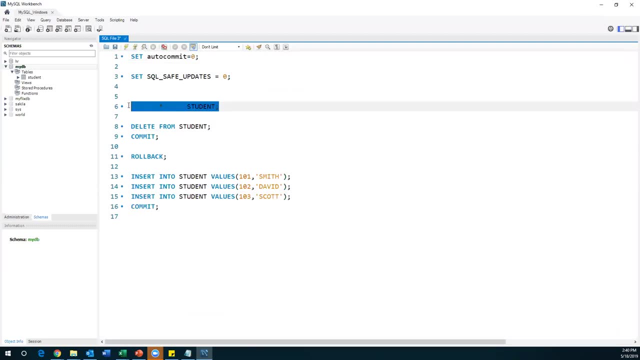 executed these steps or statements, that commit will be also executed by default. okay, so now I have done this, I am also executing my commit, so my records are permanently stored in my table. so currently I have a three records. so now I will use truncate command. so the command is truncate. ok, truncate table. 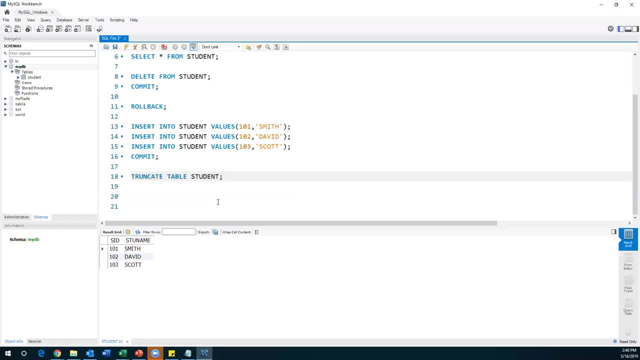 table name. I, just a student, run get table name. that's class least one and I willел throw thes in committee. table name is student. so what this command will do is this butler command will also remove the data till the stable structure is there. okay, in future you can also add more number of records. 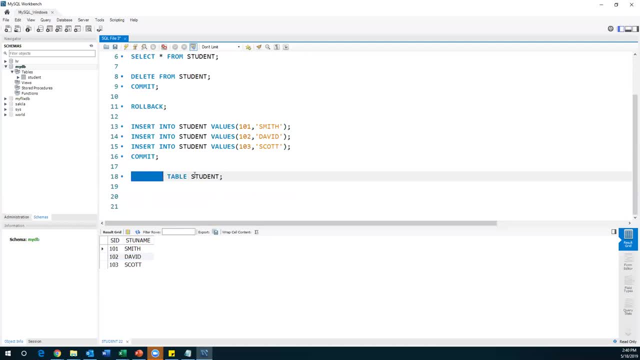 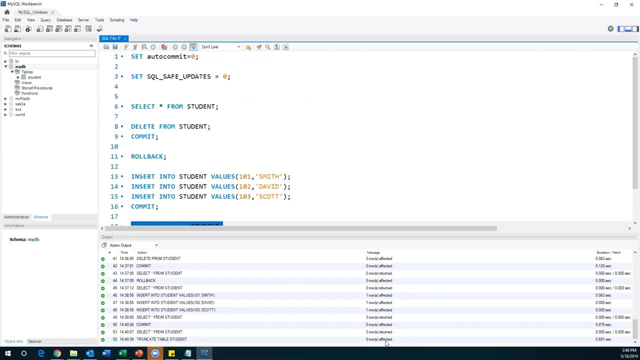 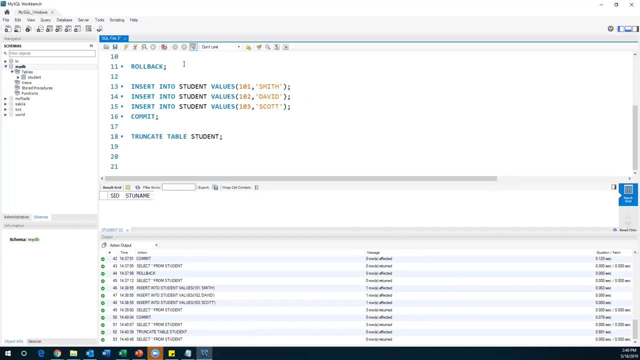 but this command will delete the data permanently. okay, so now execute this. execute it and now you can see the output. truncate table- student is successfully executed. so now, if i select star from student, you don't see any data. so even though if you do the rollback, you will not get. 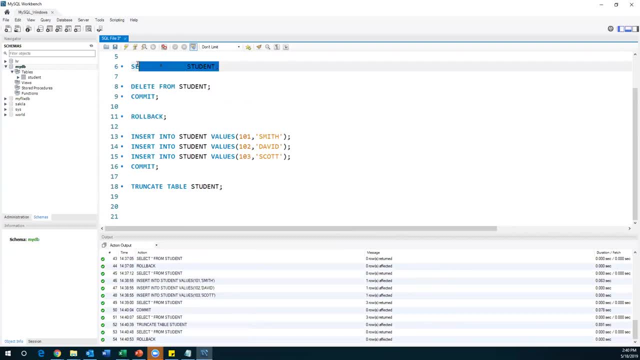 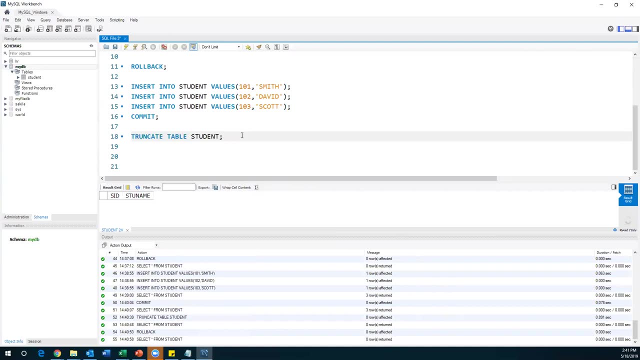 any data there. so after rollback: also, if i execute this select star from student, you don't see any data. okay, because truncate command will permanently remove the data. you cannot roll back that particular data. okay, you cannot get back the data. so that is a use of truncate command. so now we 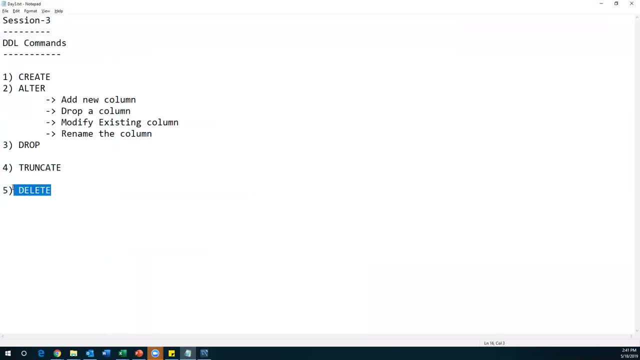 have understood what is the difference between delete and truncate. right, so delete command, truncate command will do the same job, but the only difference is delete command. if i use, i can get back the data by using rollback command, but when you do the truncate, i cannot get back the. 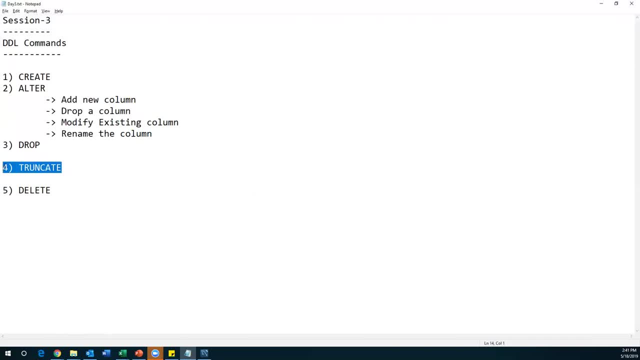 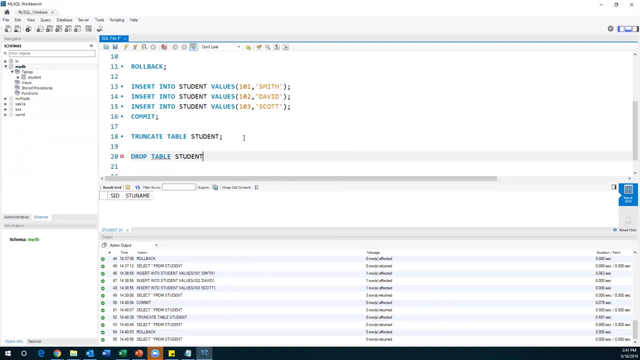 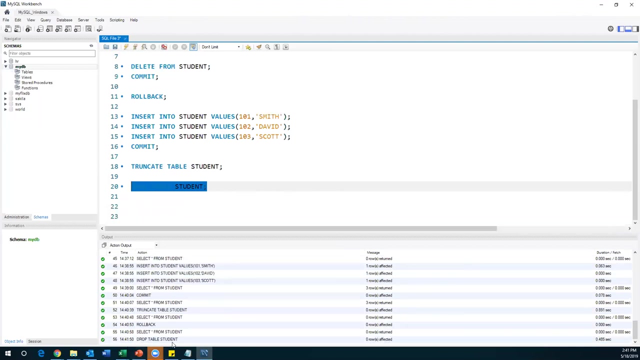 data. it is permanent change. okay, so now the drop command. so drop command will completely remove the definition itself. even the table itself will be removed. so let me use drop command, so drop table and table name. that is your student drop table table name. so this will completely drop the table. so now i have executed drop table student is done. 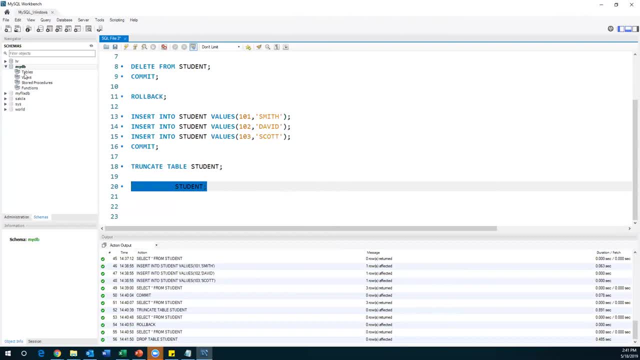 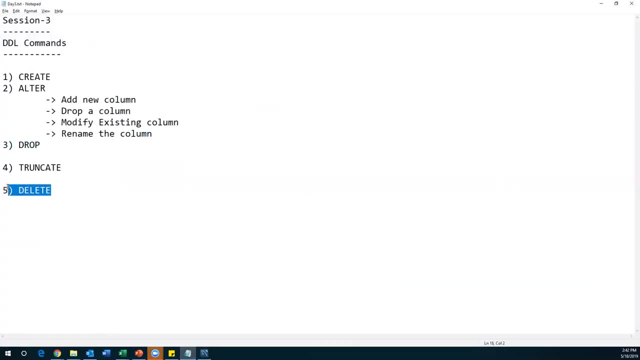 so if you see here under my db, the table is completely deleted. okay, so drop and truncate comes under the ddl commands and delete these comes under the dml command, because this works only on the data, not on the definition. okay, so now we have understood what is the difference. 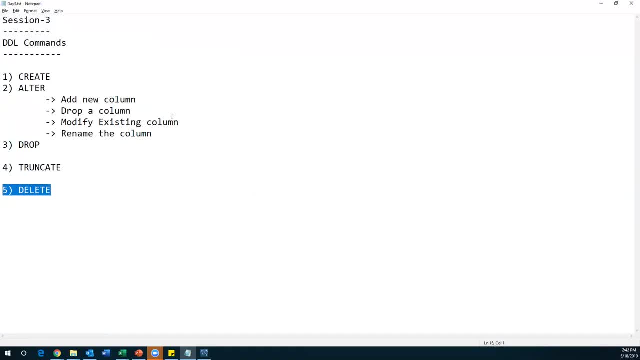 between drop, truncate and delete command. so now we have understood what is the difference between drop, truncate and delete. so drop, truncate and delete. so drop command will drop the complete table data along with the structure. and truncate will delete the complete data permanently, but still structure is present. and delete command will delete the data only, but that is a temporary. 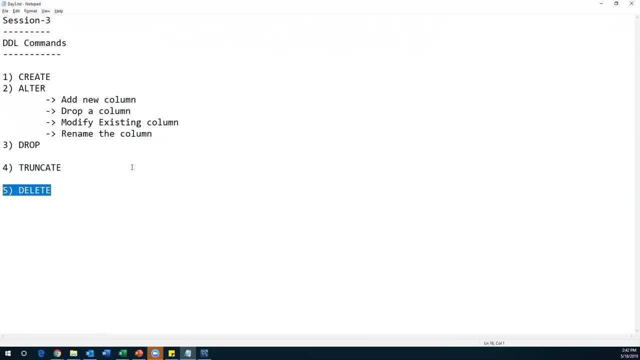 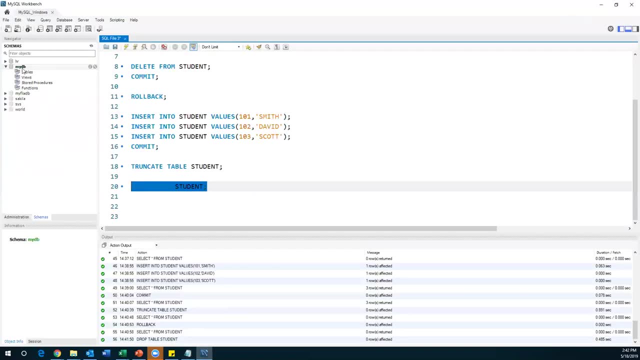 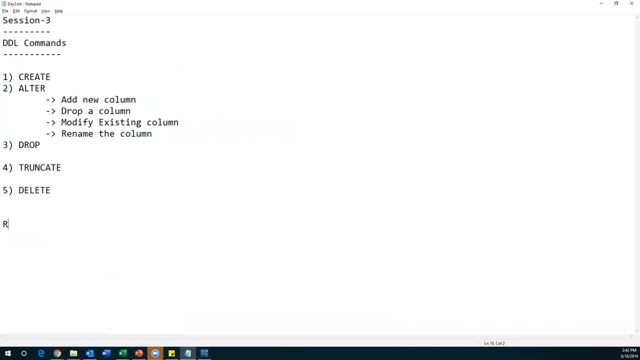 we can also roll, get back the data, okay. so now i will show you one more command. i want to rename the table. for example, let us say i have one table in my database. i want to rename it table. how we can rename it. so, renaming a table. we have seen how to renaming the column by using 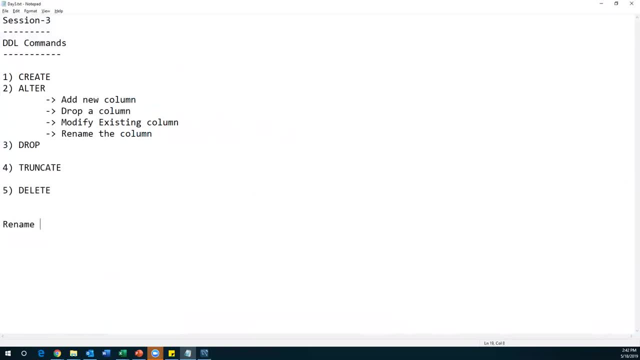 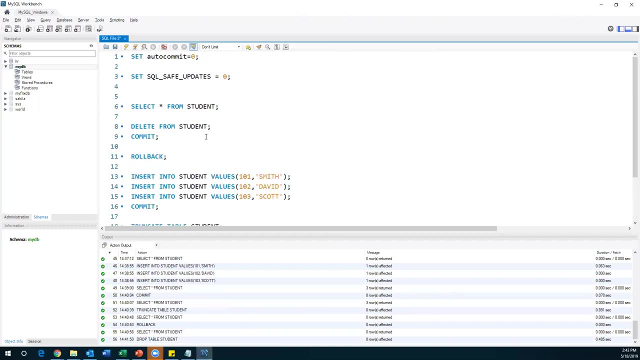 alter command. but here i'm saying how to rename a table. table name. so let me just create one more time student table. so here create, because i need to just rename the table. or you can take the any existing table. let's go for hr database. okay, so now i'll move on to the hr database. so in hr database there are multiple tables, are there? 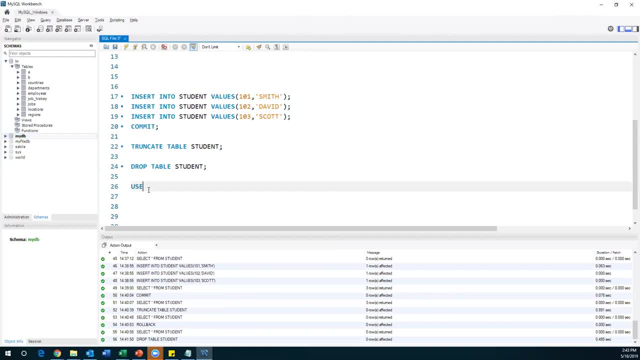 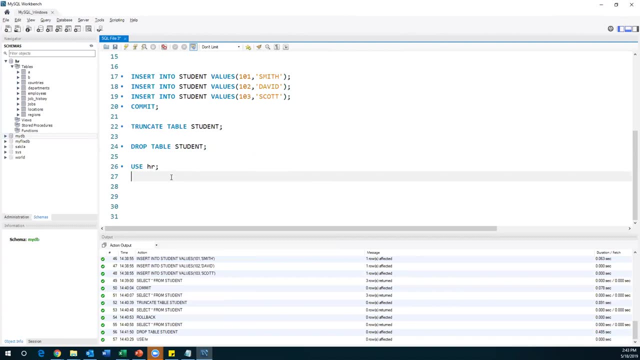 so i need to switch to the hr database by using use command. let's say use hr. so when i execute this command now i'll switch to the hr database. so now in the hr database i have multiple tables. i want to rename one particular table, okay. so for example, here i have a table called 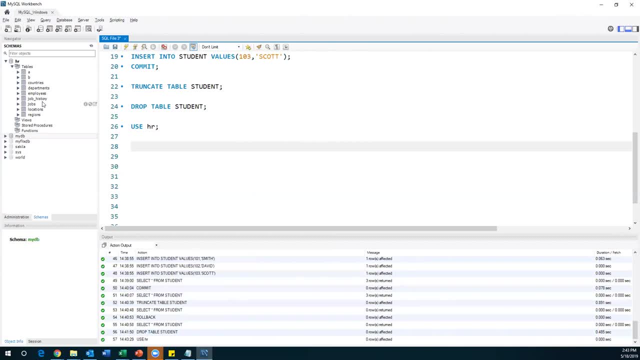 let us say, okay, jobs, so i have a table called as a jobs, so i want to rename this table. so how we can rename this table? so to rename the table we have to use a command called rename directly. rename table is a direct command. rename table and table name is the jobs. table name is the jobs and. 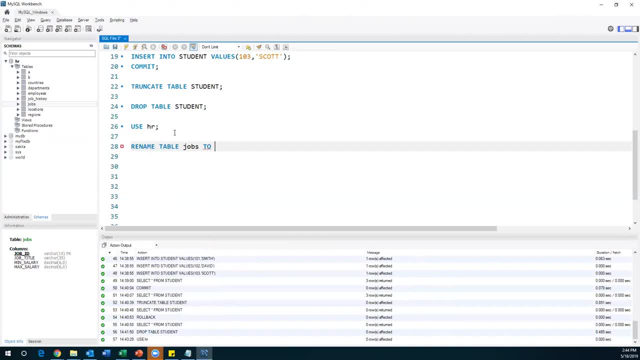 two jobs, two and the new name we have to provide. so i will say designations. okay, so rename table jobs to designation. so job is my jobs is my old name of the table, designation is a new name of the table. so once we rename the table, the data structure, table structure.